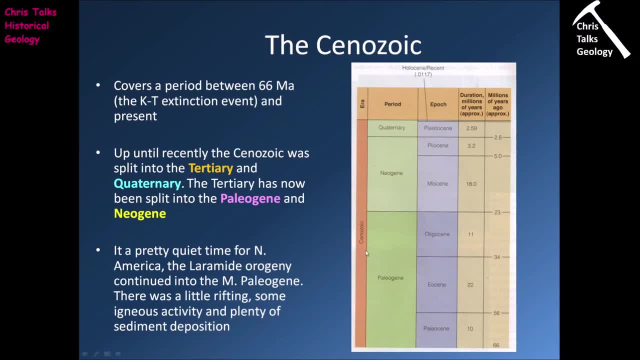 Now to be clear, the Cenozoic itself is an era. So in terms of the eras that we have in the geologic timescale, the Cenozoic is actually quite small. So at 66 million years it's actually smaller than the Cretaceous period. 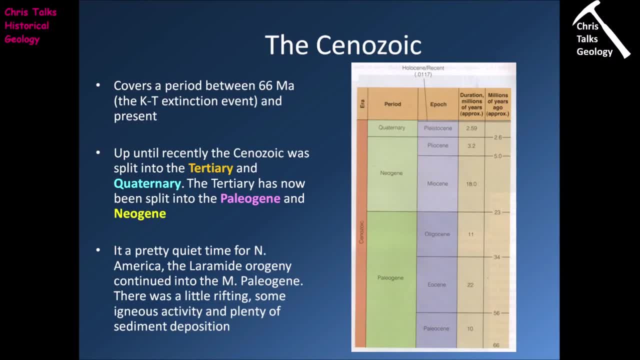 So that shows you that from a geologic point of view, it's not a huge amount of time. Now, up until recently, the Cenozoic was split into the Tertiary and the Quaternary. The problem was: is that, using that? 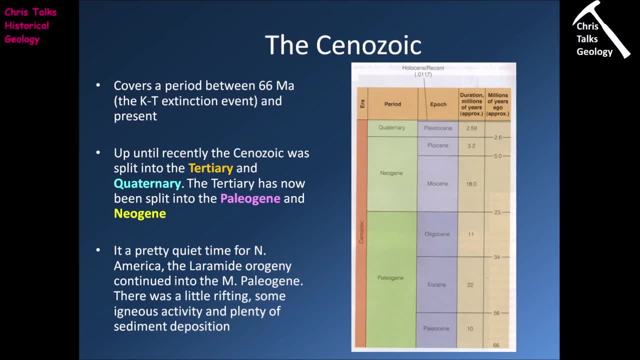 that system. the Tertiary essentially represented a period of time from 66 million years ago to 2.6 million years ago, So it's about 63 million years, which is a pretty large chunk of time for a single period. So it was decided that, you know, the Tertiary should be split into two smaller units, and these smaller units are termed the Paleogene and the Neogene. 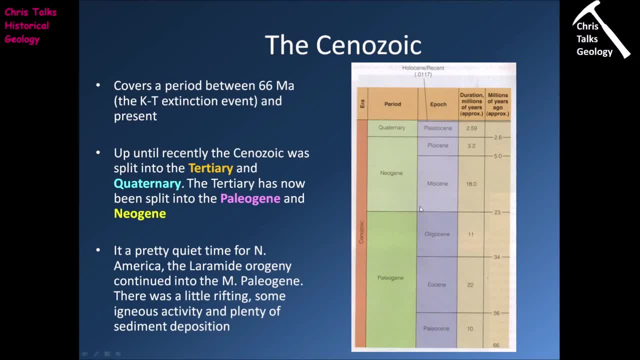 So the Cenozoic has three periods: the Paleogene, the Neogene and the Quaternary. Now, when we're talking about the Cenozoic, we don't actually talk about the periods that much. We actually prefer to use the epochs instead. 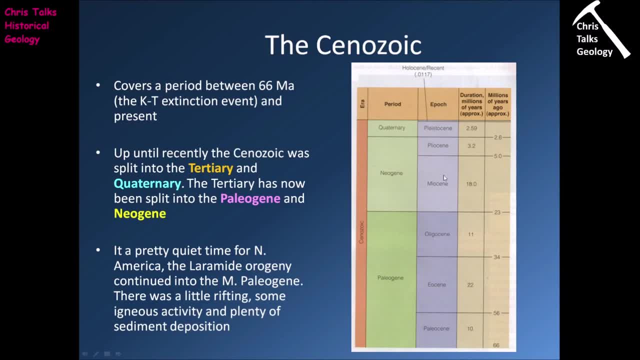 So, in terms of the epochs, there's the Paleocene, the Eocene, the Oligocene, the Miocene, the Pliocene, the Pleistocene and the Holocene. Now, the reason we prefer to talk about the epochs is because they're smaller units. 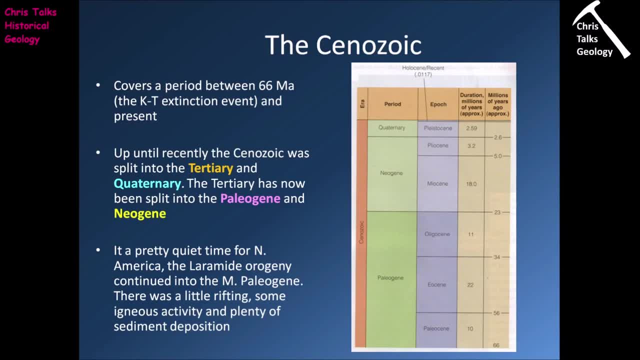 They just mean that we can be a little bit more exact in you know about what portion of the Cenozoic we're talking about. It just makes things a little clearer. Now, in terms of geology, during the Cenozoic for North America it was actually relatively quiet. 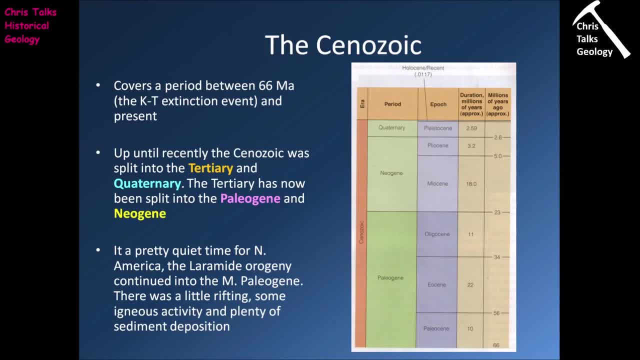 So we had subduction continuing along the west coast of North America until the middle Paleogene. We had a little bit of rifting taking place, We had a bit of igneous activity and obviously we had plenty of sediments being deposited all over the place. 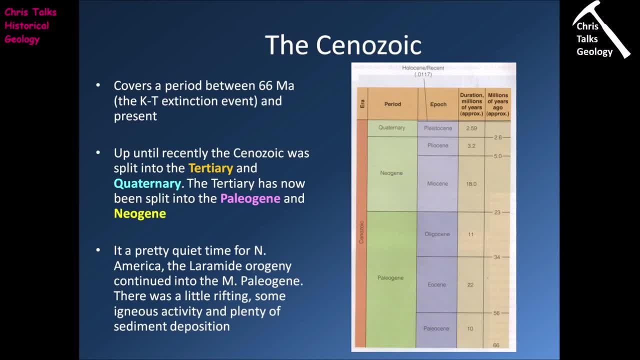 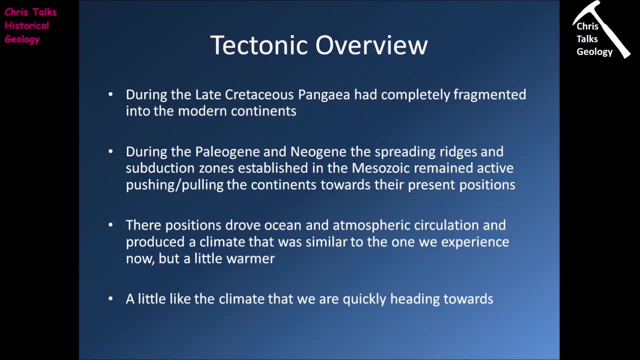 But on the whole it's actually a relatively quiet period of geologic time for North America. So let's start by doing a quick tectonic overview. So during the late Cretaceous, Pangaea had completely fragmented into the modern continents as we know them. 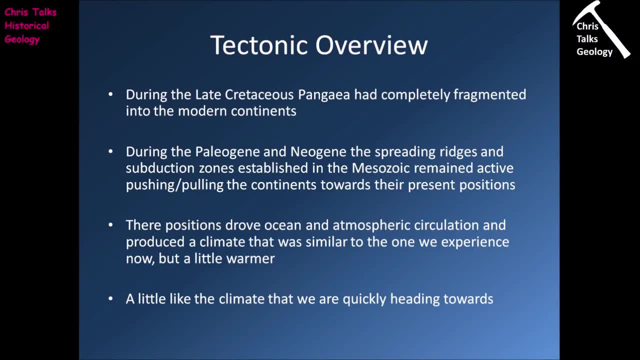 Now, during the Paleogene and the Neogene, the spreading ridges and subduction zones that have been established in the Mesozoic remained active and they started to push and pull the continents towards their present positions. Now, as we discussed, the changes in the position of the continents obviously have an effect on ocean circulation and atmospheric circulation. 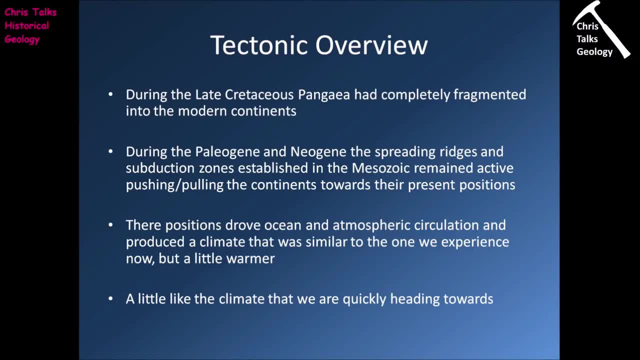 And so that obviously produces changes in the geological order. There are changes in climate, But at the same time, we need to remember that for much of the Cenozoic, the global climate as a whole was warmer than it is now, So the climate in general would actually be more like the climate we're heading towards now, courtesy of global warming. 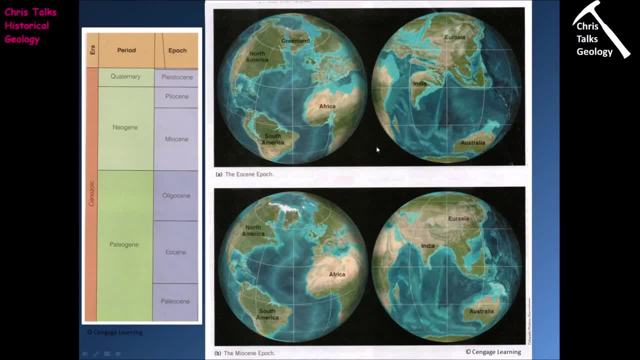 So in terms of the distribution that we have. so at the top we have the distribution of the continents for the Eocene and at the bottom we have the Miocene. So the Eocene is down here. So essentially it's the middle Paleogene. 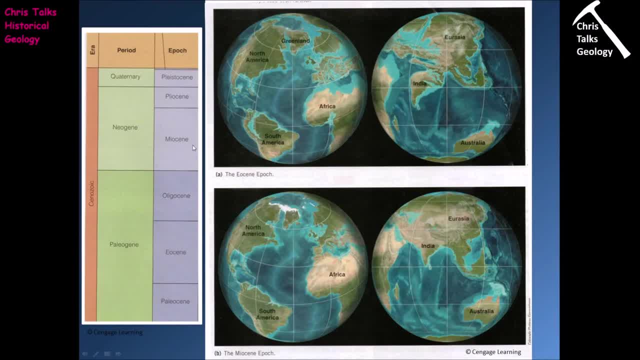 And the Miocene is up here. It's the lower and middle Neogene. So what can we see? Well, to begin with, we can see that we have the modern continents in approximately their modern position, So everything looks kind of familiar. 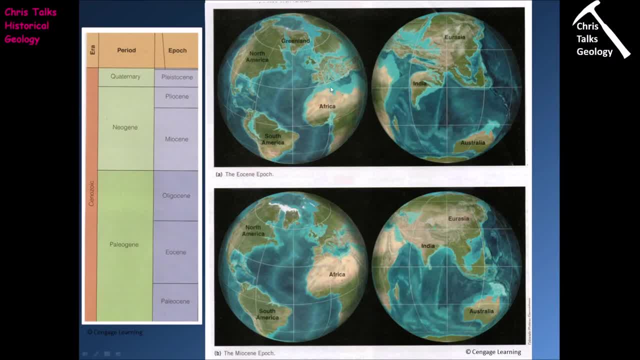 Now we can see that during the Eocene there was definitely a marine transgressive event going on. You can see large portions of Africa are underwater. A substantial portion of South America is underwater, But we can see where the continents are located. 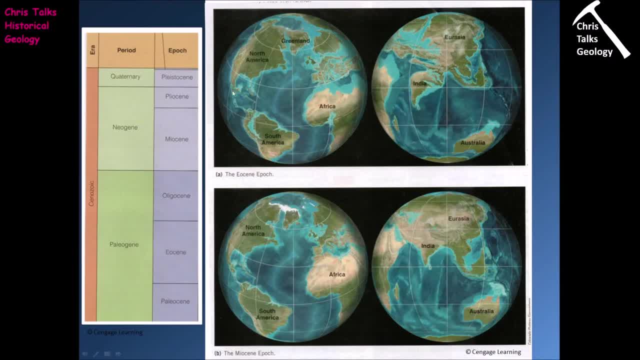 And obviously we know where they're going to end up. We can see also at this point that South Africa is going to end up. We can see also at this point that South America and North America aren't joined together. We can see that Africa hasn't made contact with Europe yet. 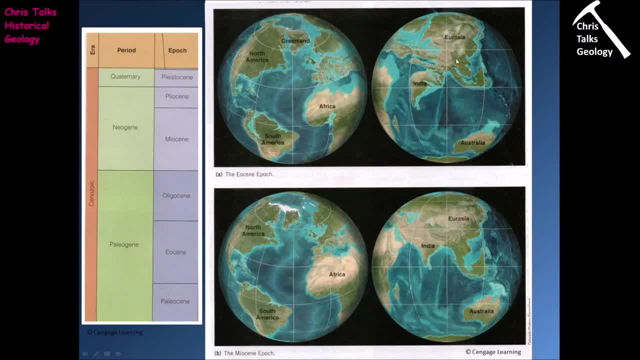 And India is still making its way to Asia as well. Australia is only just separated off from Antarctica and it's beginning to work its way northwards. So, if you remember, there's a subduction zone that's running all the way along the southern margin of Asia and along the southern margin of Europe here. 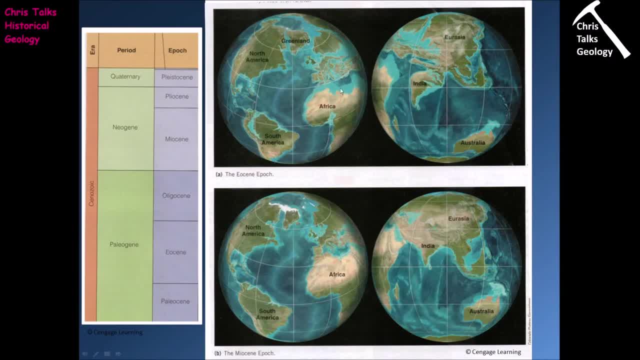 And that subduction zone essentially is helping to pull Africa northwards And it's helping to pull India northwards as well. And we know what's going to happen: There's going to be a collision. The collision between Europe and Africa essentially is going to produce the Alpine Orogeny. 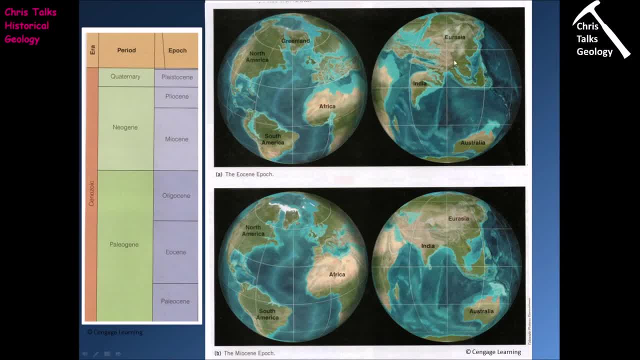 And the collision between India and Asia is going to produce the Himalayan Orogeny. Now, because Africa and India and South America haven't made contact yet with the other continents, it means essentially there's a channel through which water can circulate essentially around the entire Earth. 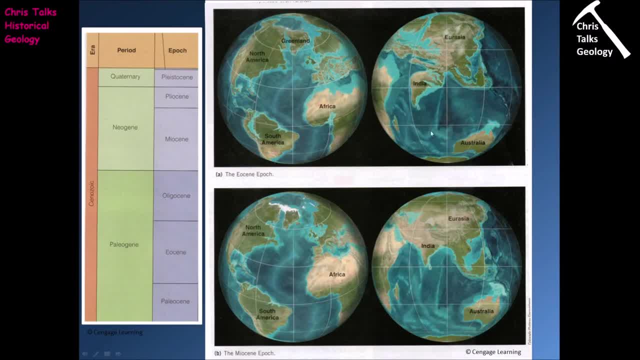 So the water can come from. you know the modern day Indian Ocean. slash what's left of the Tethian Ocean Basin So that hot water can come from this area. It can travel along the northern edge of Africa into the Atlantic. Then it can go from the Atlantic into the Caribbean, into the Pacific and then back into the Indian Ocean. slash Tethian Ocean. 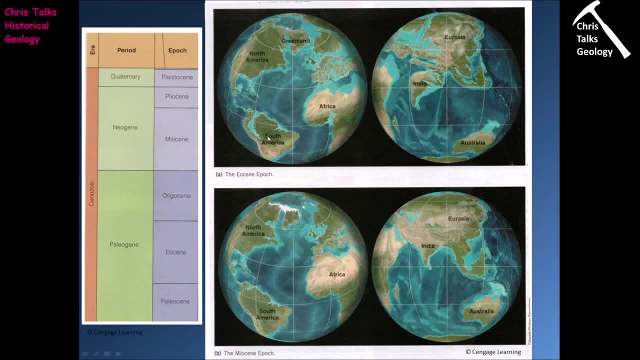 And so it meant that during the Eocene there was still the capacity for full circulation of seawater. you know relatively easily. Now, by the time we've made it into the Miocene, you can see that South America and North America are just about to make contact. 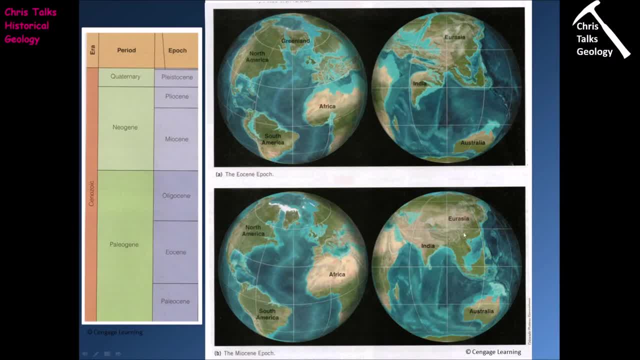 Africa and Europe have begun to interact with each other. India is now slammed into Asia, And so this means this channel for water circulation is now closed up, So we can't get nice warm water from the Indian Ocean moving into the North Atlantic, for instance. 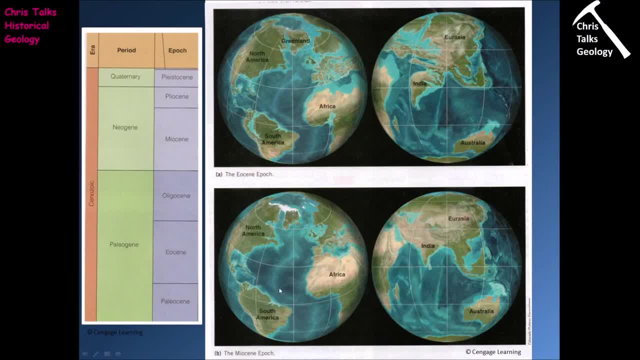 So that's obviously going to have, you know, a noticeable effect on climate. So by the time we're into the Miocene, you can quite clearly see that the continents are approaching their current positions. But you will notice there are some differences. 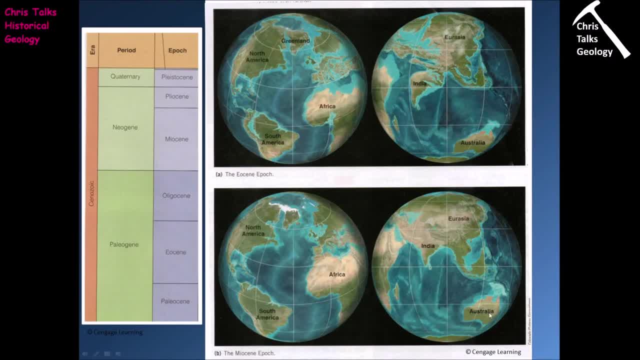 As I said, South America and North America are in contact. We can see that Australia is still working its way north And we can see that Southeast Asia hasn't quite taken on its more modern look. We can see the Philippines, Indonesia and, essentially, the Thai Peninsula are all joined together as one unit during this time period. 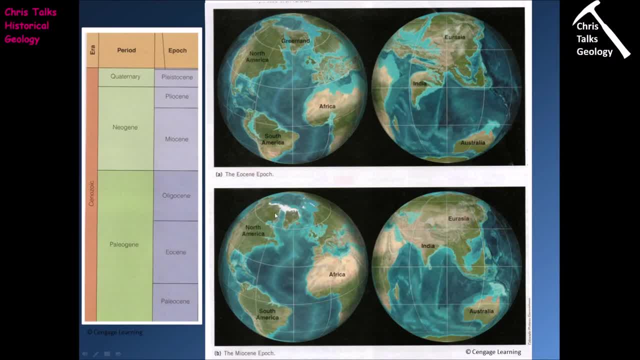 We'll also notice that as we transition from the Eocene to the Miocene, we begin to see indications of ice caps. So we can see some ice caps forming here in the north, towards the North Pole, And we can just see some ice caps forming down here towards the South Pole. 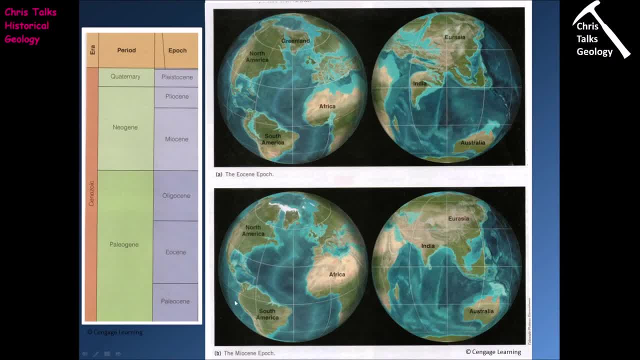 And essentially this is a general picture. This is a general trend that we see as we're moving from the Cenozoic. At the start of the Cenozoic, we start with higher temperatures, similar to those of the Cretaceous. 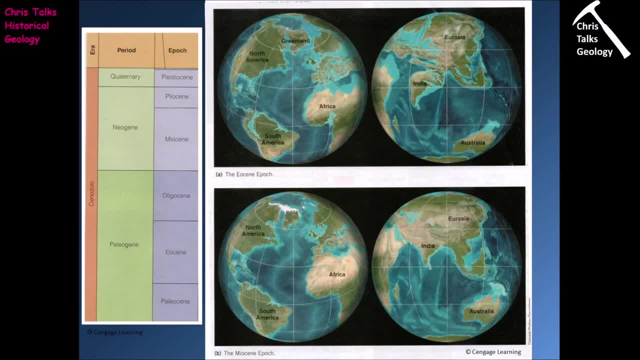 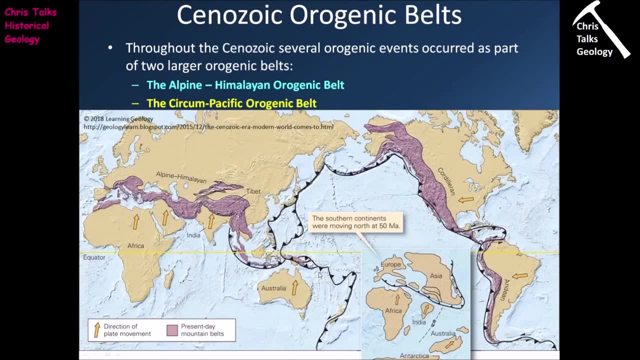 And then, as we move towards the present day, on the whole we have a gentle decrease in global temperatures, leading to more ice cover at the poles. Okay, so let's talk about the global orogenic belts in the Cenozoic. There are two main orogenic belts that we have to talk about. 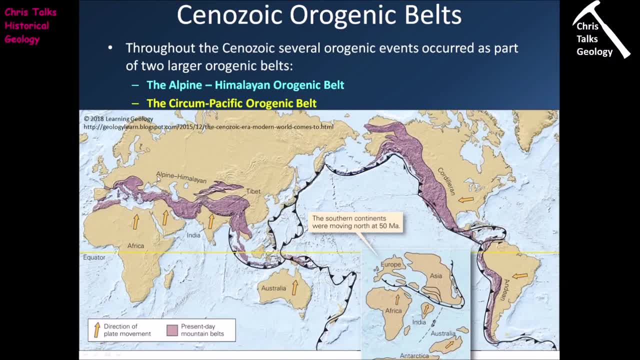 The first is the Alpine-Himalayan orogenic belt. So the Alpine-Himalayan orogenic belt starts over here in northwestern Africa, so over here in Morocco. It continues all the way through southern Europe into the Middle East and then essentially into what we would refer to as the Himalayas, the Tibetan Plateau. 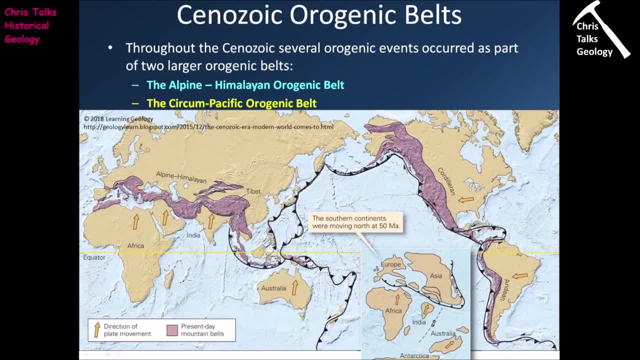 Then it continues down the Thai Peninsula and into what we would refer to as Indonesia now. So you can see, we have a more or less continuous chain of mountains coming all the way over here, from Morocco, All the way over here to Indonesia. Now these mountains are the result of the northward movement of Africa, the Arabian Peninsula and India and its interaction with Europe and Asia. 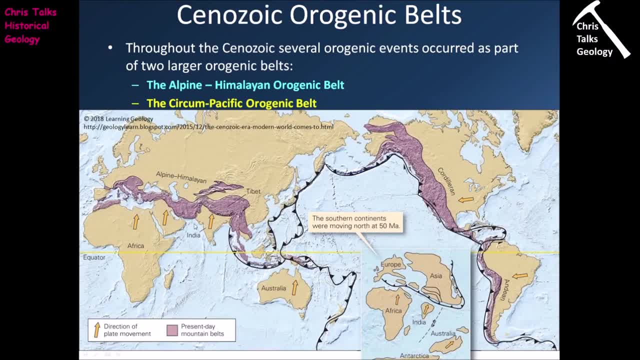 And, of course, as we know, this is due to the fact that there was a subduction zone that was running along the southern margin of Europe and Asia And that helped to pull these pieces of continental crust northwards Now in terms of the circum-pacific belt. 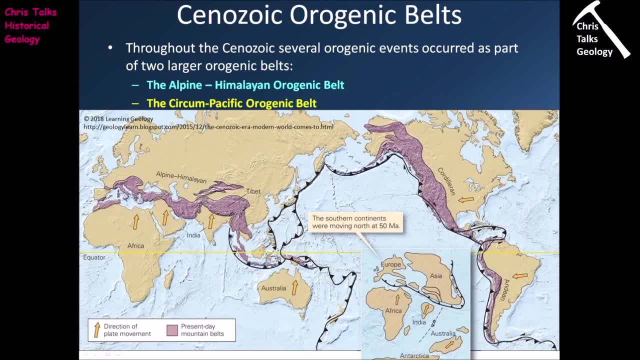 we have a belt of mountains that starts all the way over here in the southern tip of South America, continues up the west coast of South America, Central America and North America, continues across the northern Pacific via the Aleutian Islands and then it comes down the western side of the Pacific. 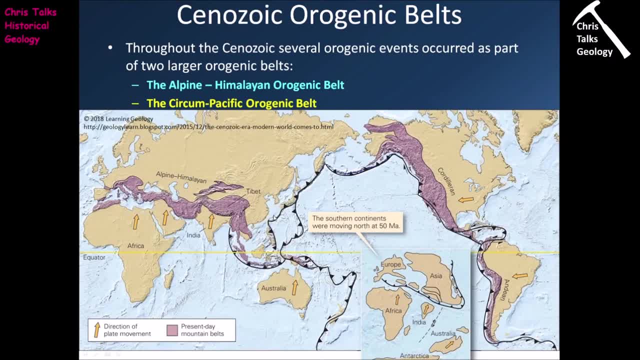 So we have a trench that comes down towards Japan, Then it splits. We have one limb that comes down here towards the Philippines, one limb that essentially is here in the middle of the Pacific Ocean itself, And then we come around here and then it comes down through Papua New Guinea. 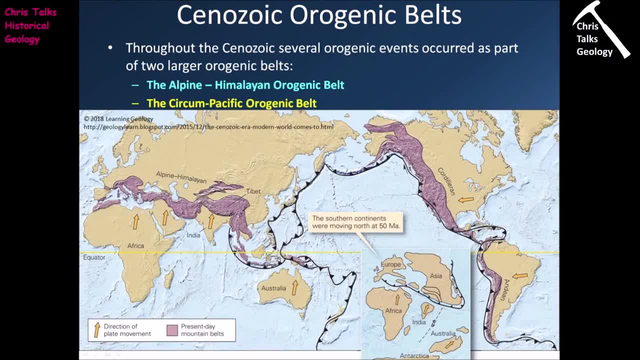 Loops around via Fiji and Tonga and then comes down towards New Zealand, And so in this case, this particular orogenic belt is related to ocean-continent and ocean-ocean subduction. So in the case of the Alpine Himalayan belt, we have a mountain range that's resulting, on the whole, from continent-continent collision. 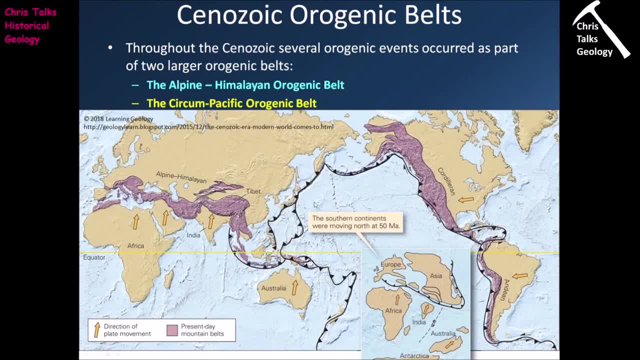 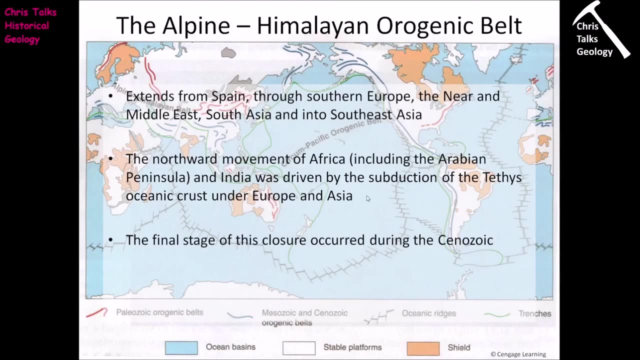 In the case of the circum-pacific orogenic belt, we have a system that's dominated by ocean-continent and ocean-ocean subduction, So we have different types of plate convergence, essentially producing these large chains of mountains. So let's start by talking about the Alpine Himalayan orogeny. 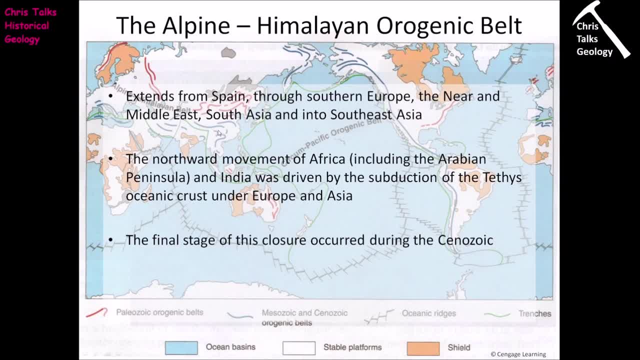 So it extends from Spain through southern Europe, the Near and Middle East, into South Asia and then eventually into Southeast Asia. So of course, the Himalayan Alpine orogeny is the result of the northward movement of Africa and India. 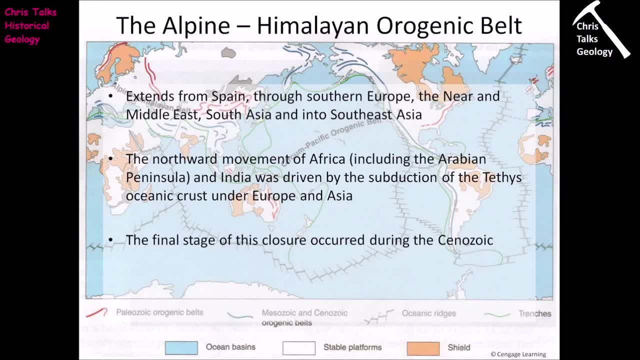 And, of course, as we know, there was that subduction zone. That's what's helping to move them northwards And it leads to, you know, the collision of Africa and the Arabian Peninsula with Europe and the Middle East and, of course, the collision of India with Asia. 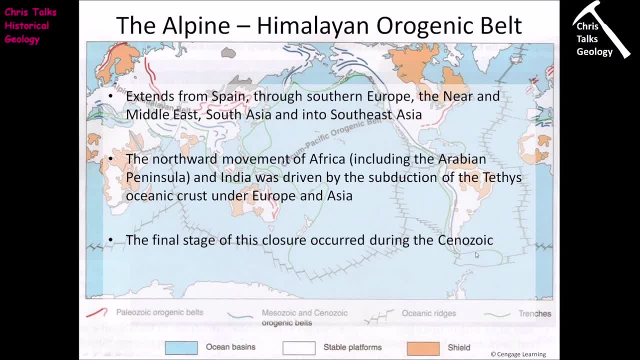 Now the final stages of this closure event occurred during the Cenozoic and it's actually still going on now. So Africa is still moving northwards, so it's still colliding with Europe, and India as well is still moving northwards as well. 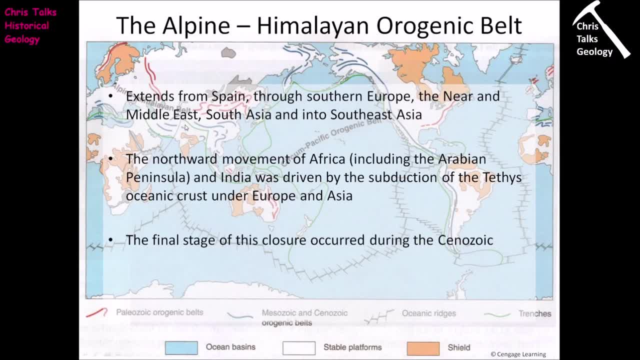 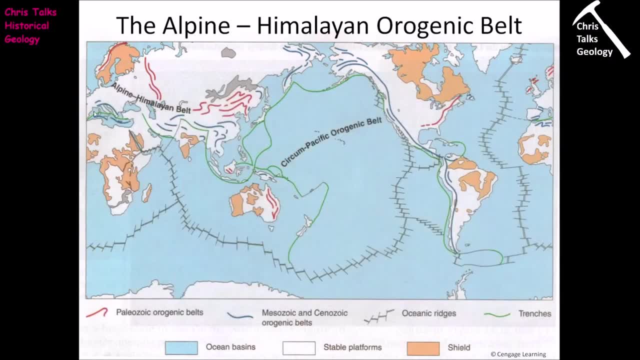 So the Alpine orogeny and the Himalayan orogeny are still currently active events, So you can see the band here running all the way from well, there's Spain over here, actually running all the way from Spain all the way across southern Europe, Middle East and then into South Asia. 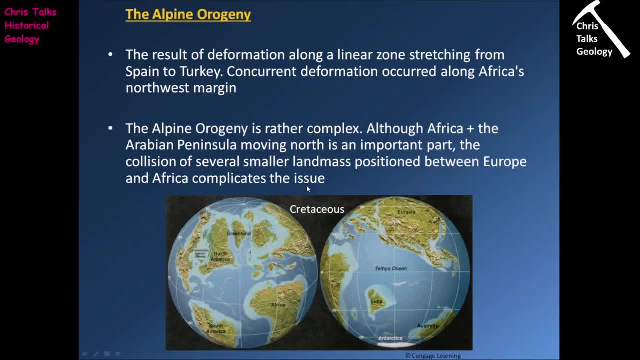 and then eventually all the way down into Southeast Asia. So in terms of the Alpine orogeny itself, it's the result of deformation along a linear zone that stretches from Spain to Turkey primarily. We get concurrent deformation as well on the other side. 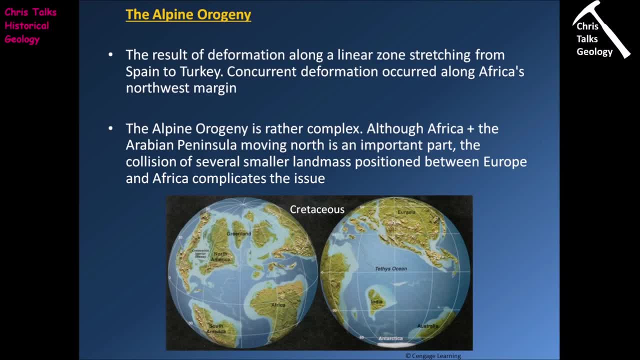 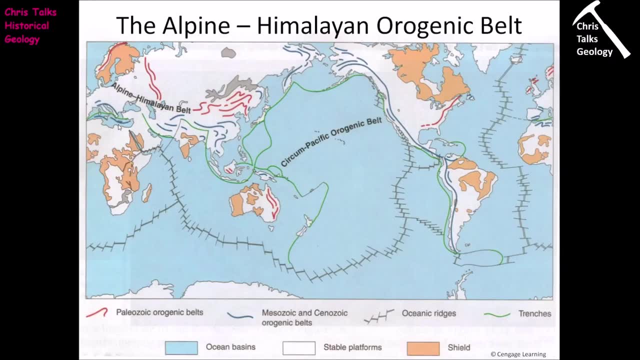 So essentially the northern coast and northwestern coast of Africa. So obviously when we have a collision- if I just go back to the previous slide here we not only have the deformation caused by Africa hitting Europe, we obviously have the deformation caused by Europe hitting Africa. 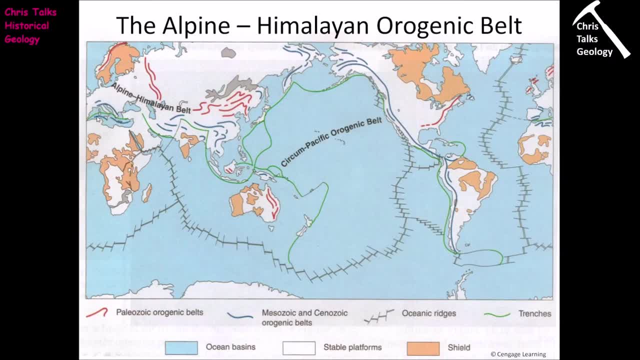 So we get you know deformation on both sides. Most of it, though, is focused on the northern side of the collision, which, essentially, is where Europe is located, So most of the surface expression of the collision is going to be visible on the European side. 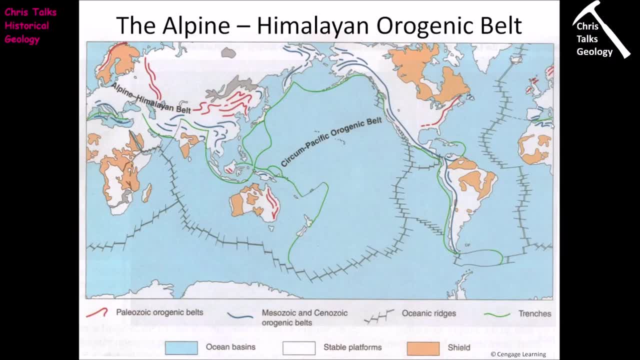 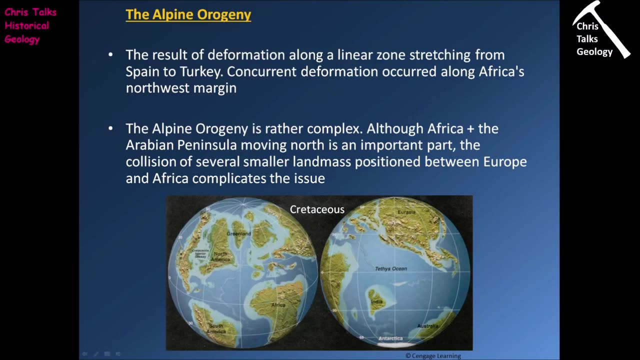 We do have a little bit of it visible in Africa, so of course we have the Atlas Mountains of Morocco. That's a surface expression of the collision, but the vast majority of the deformation has been focused into the European continent, So the Alpine orogeny itself is rather complex. 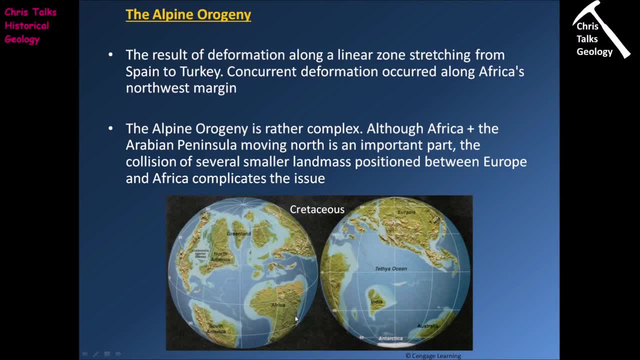 So if we look at this map down here for the Cretaceous, what you'll notice is that in between Africa and the main mass of Europe, you'll see there are several land masses, and these land masses are going to consist of pieces of continental crust. 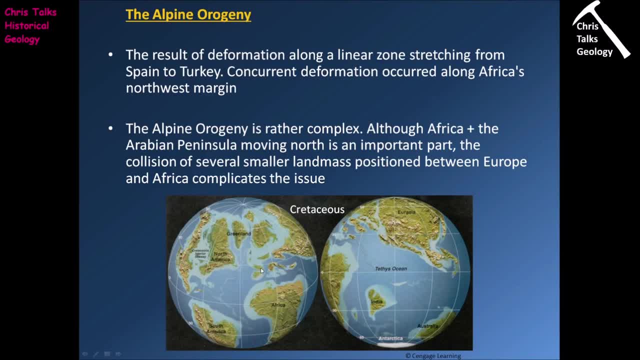 that will go to make Spain and Portugal, southern France, Italy and some of the Balkan states, Greece and bits of Romania and Hungary, etc. So as Africa moves northwards, what's going to happen is these little pieces of continental crust are also going to be pushed northwards. 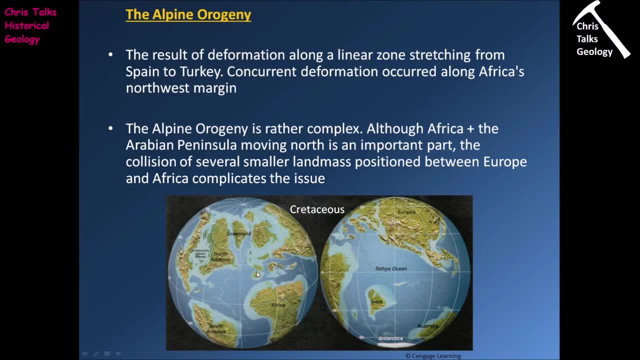 and they're going to hit Europe. So essentially, each one of these microcontinents hitting Europe is going to produce its own small mountain range And, of course, all of these individual events are going to be tied together and essentially put under the umbrella of the Alpine orogeny. 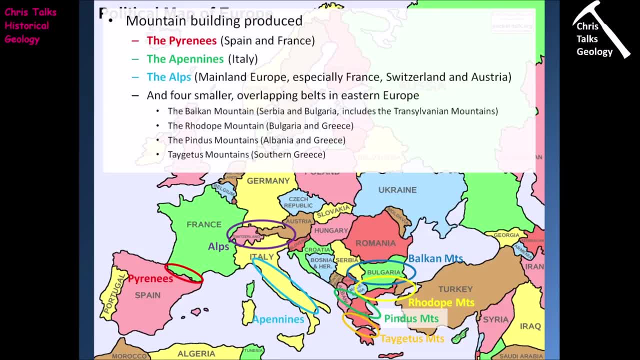 So if we look at the Alpine orogeny and if we just look at a map of Europe, we can see that it actually consists of several individual events. So, for instance, we have the Pyrenees. The Pyrenees sits between Spain and France. 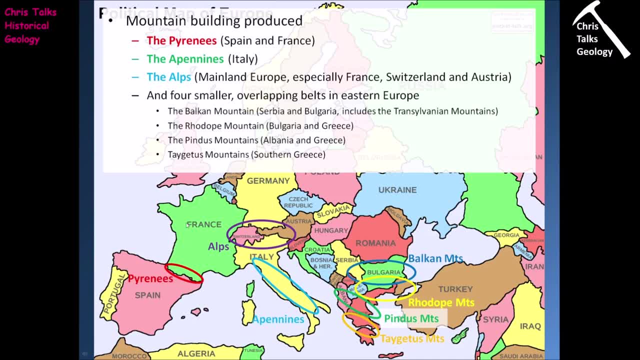 and this was produced by the impact of the Iberian Peninsula along the southern margin of what is now modern-day France and that produces the Pyrenees. We obviously have the Alps themselves. That's produced by the collision of Italy with the mainland. 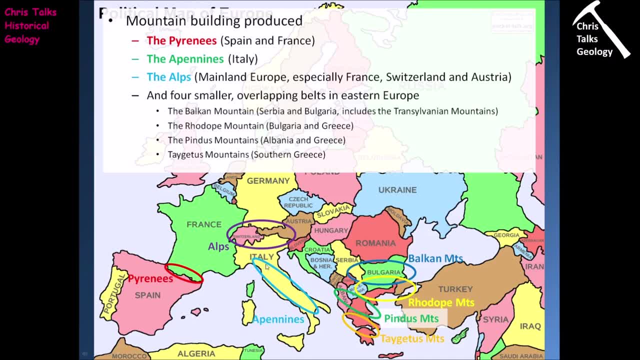 a massive mass of Europe. We also have the Apennines forming along the length of Italy. That's a result of the deformation of Italy by the northward movement of Africa. And then we have a set of smaller mountain ranges over here. You can see they all overlap with each other. 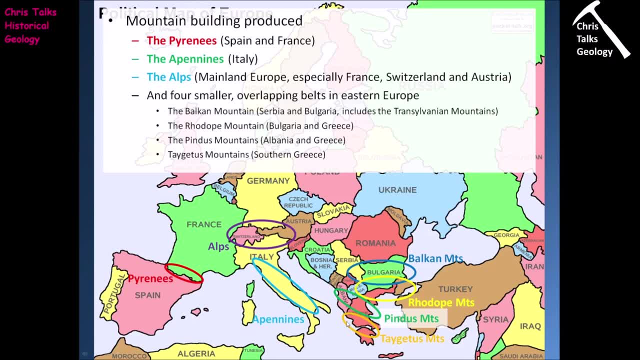 So these have all been produced by small pieces of continent slamming into Europe one after another. So we have the Balkan Mountains. That's mostly focused around Bulgaria and Serbia. We have the Rhodope Mountains. Those are mostly focused in northern Greece, Macedonia and southern Bulgaria. 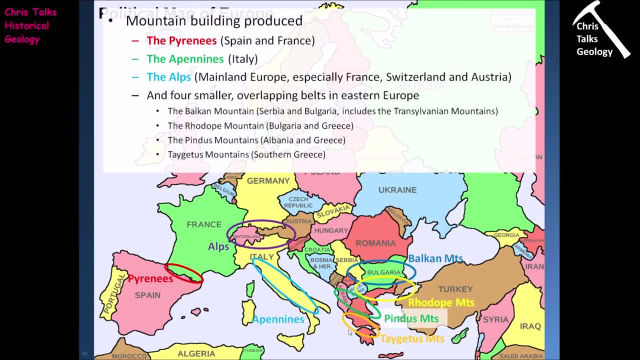 We have the Pindus Mountains- That's mostly northern Greece and Albania- And the Tigritus Mountains. Those are mostly in southern Greece. That's the Tigritus Mountains- I do apologize for my pronunciation there. So each one of these mountain ranges represents the impact of a small piece of continental crust. 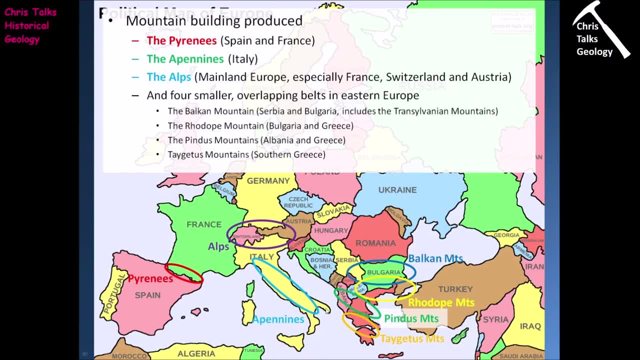 along the southern margin of Europe as Africa was moving northwards, And all of these individual impacts are essentially considered to be part of the larger alpine orogeny. So even though the Alps themselves only cover this small area marked out here in purple, 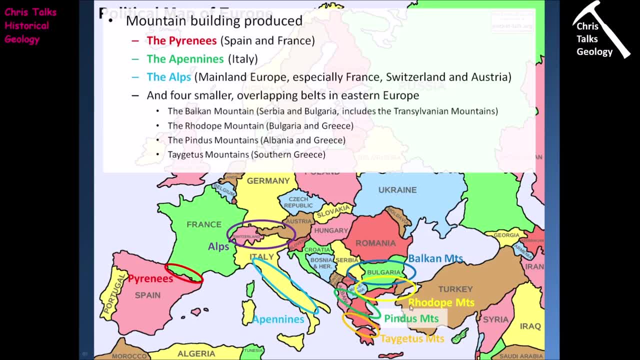 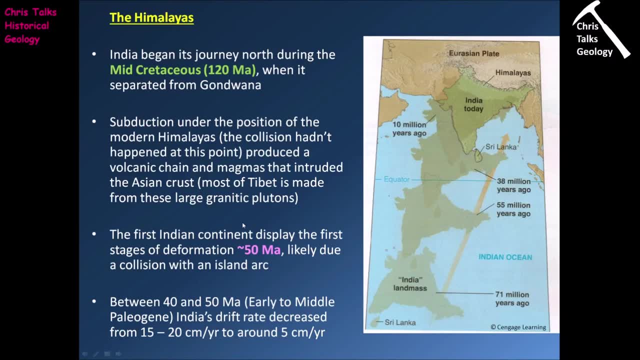 the entire orogenic event itself is referred to as the alpine orogeny. So obviously, at the other end of the orogeny we have the formation of the Himalayas. So India began its journey northwards during the mid-Cretaceous. 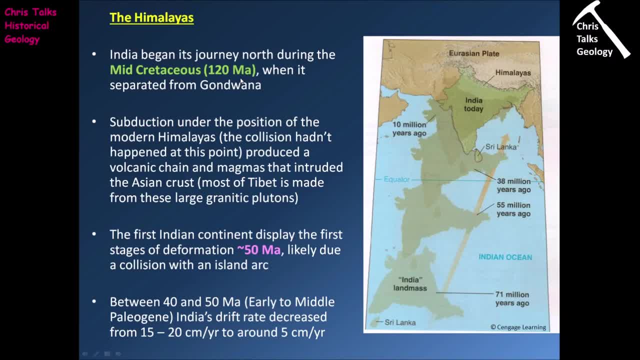 So about 100 million years ago, 120 million years ago, the continent of India rifts off what's left of the remnants of Gondwana And it begins to move northwards, essentially across what was the seafloor of the Tethys Ocean. 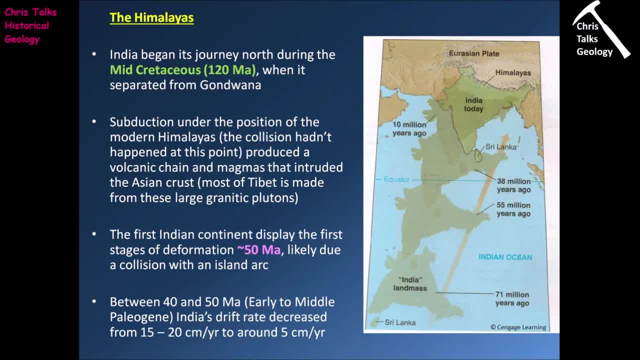 Now, this northward movement was driven by a subduction zone located along the southern margin of Asia- Essentially, the position of it would have been approximately equivalent to the modern-day Himalayas- And, of course, this subduction zone starts to pull India in the north. 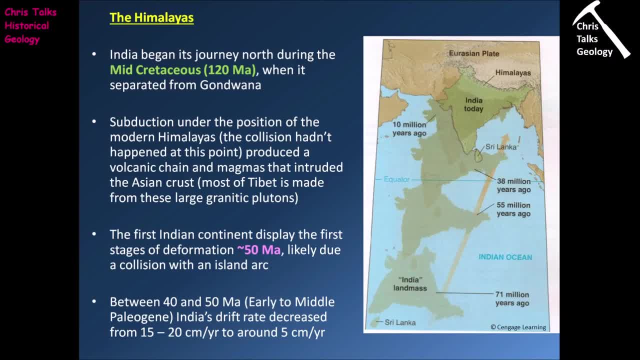 Now, before the impact actually occurred, we had a situation where we had the ocean floor of the Tethys Ocean subducting underneath Asia, And so this actually meant that before India hit Asia, there was already a set of volcanically active mountains present along the south coast of Asia. 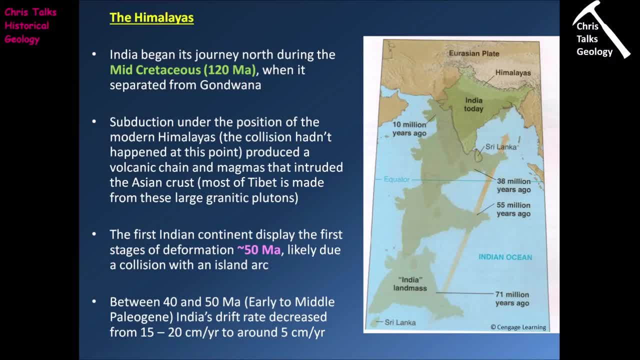 a bit like the modern-day Andes, And so this means the area which is now the modern-day Himalayas was already mountainous, very badly deformed, full of volcanoes and therefore obviously full of intrusions below the surface as well. And then, later on, India comes in. 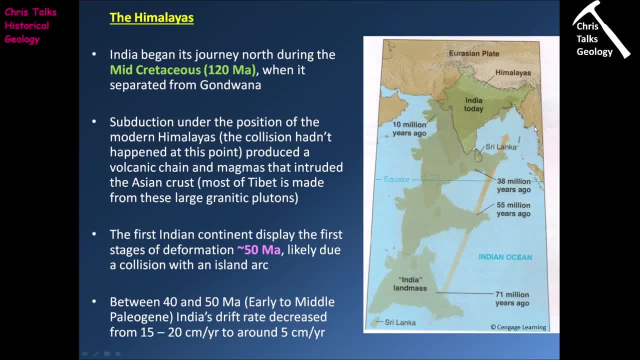 So for a long period of time this southern margin of Asia was an ocean-continent convergent boundary. And then, eventually, India will slam into Asia and produce a continent-continent convergent boundary, which will produce the Himalayan Mountains. Now the Indian continent displays the first stages of deformation approximately 50 million years ago. 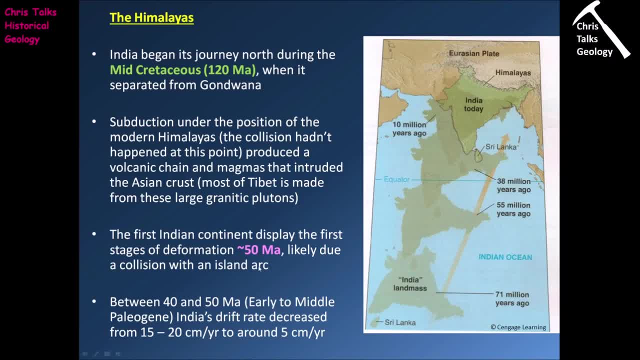 I apologise for mucking up that sentence there. So now the first indications of deformation aren't actually due to India hitting Asia. It's probable that in between India and Asia about 50 million years ago there was a small island arc, And so about 50 million years ago India runs into this island arc and we begin to see the deformation. 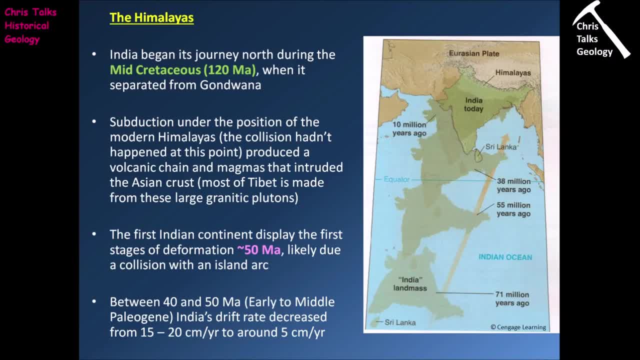 which results from India smacking into this line of volcanic islands, And so that's the first indication, That's the first stages of deformation that we see on the Indian continent Now, between 40 and 50 million years ago. so that's the early to middle Paleogene. 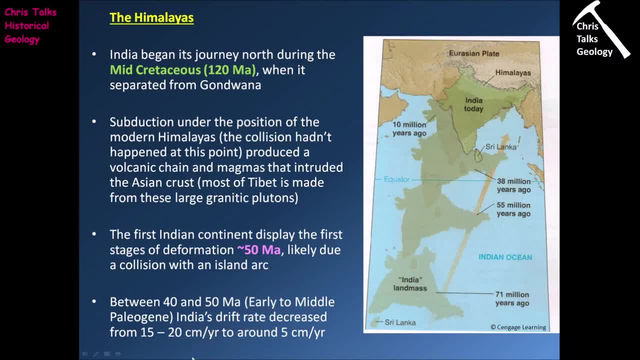 we begin to see India's drift rate decrease from about 15 to 20 centimetres a year to around 5 centimetres per year. So one of the things that happens is about 80 million years ago. the rate at which India is moving northwards suddenly accelerates a lot. 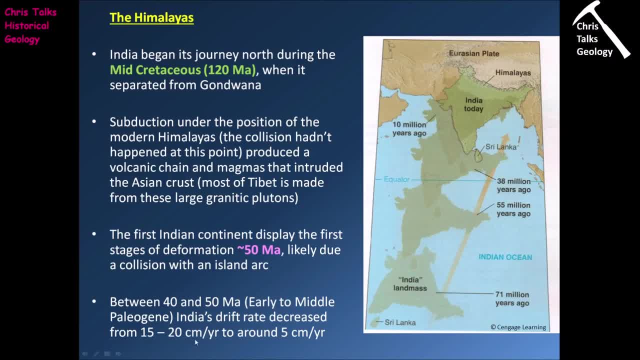 So a movement rate of about 15 to 20 centimetres a year is very, very fast. So for comparison, the Atlantic is opening up at a rate of about 2.5 centimetres a year. So the movement of India northwards from about 80 million years ago to about 40 or 50 million years ago. 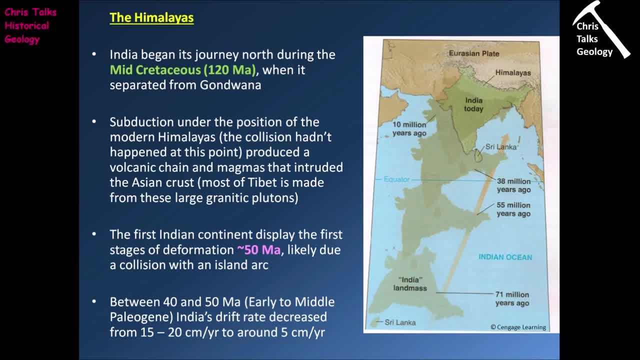 so a period of about 40 million years is very, very fast. So 80 million years ago, India accelerates to about 15 to 20 centimetres a year. It's moving northwards. And then, about 40 to 50 million years ago, we all of a sudden see this rate of movement decelerate. 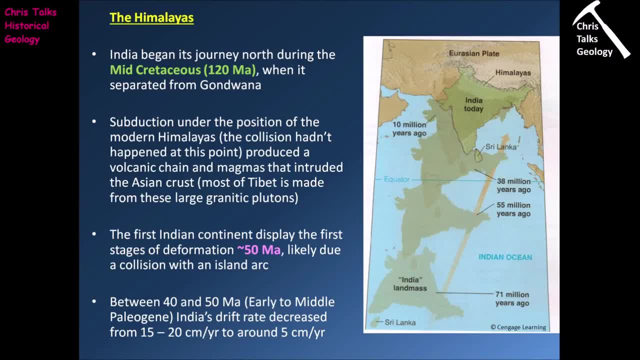 It decelerates very, very quickly, And so this is telling us now that India is beginning to interact with the main mass of Asia, And so that means essentially, as India begins to interact with Asia, of course there's a collision between these two very, very large pieces of continental crust. 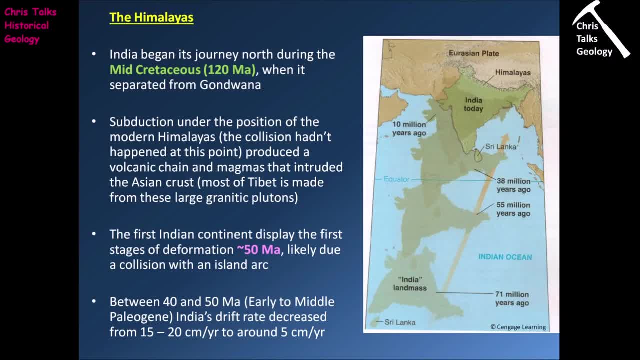 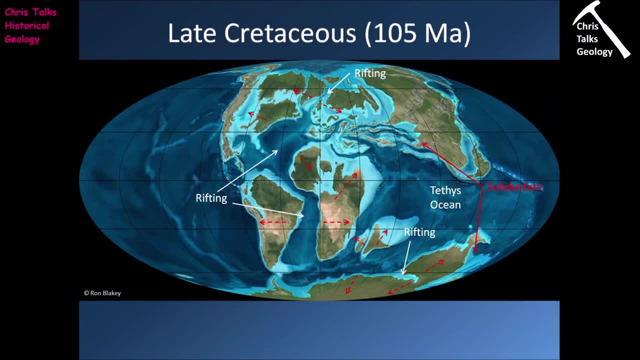 and that's of course, going to slow India down. So if we look at the map here, we can see the situation in the late Cretaceous. So at the moment we are most interested in what's going on, What's going on here with India. 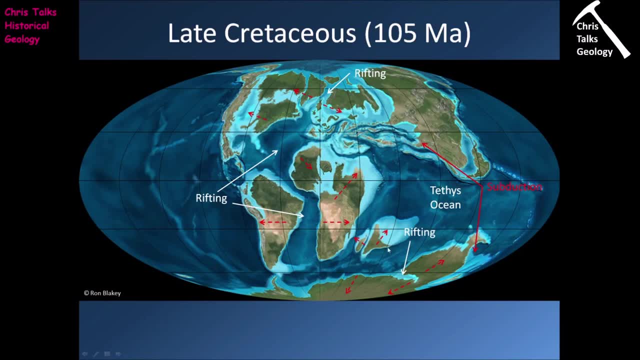 Now the one thing I will say is: take a note that this area of exposed land here is approximately equal to the size of modern-day India. But along the northern margin of India, you can see here there was a continental shelf And of course this continental shelf is going to be covered in marine sediments. 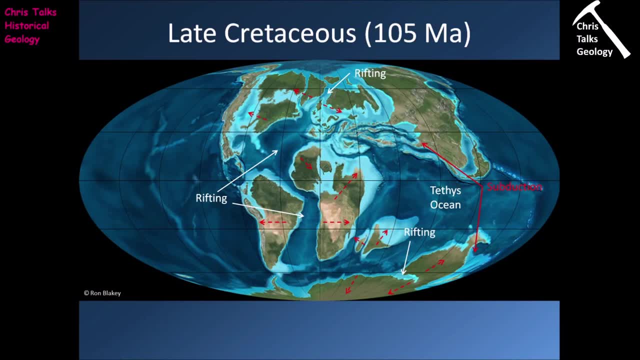 You're going to have marine sands, marine muds and carbonates And these rocks are going to be compressed and deformed and they're going to become part of the Himalayan mountains. In terms of the subduction zone there, it is running along the south coast of Asia and Europe. 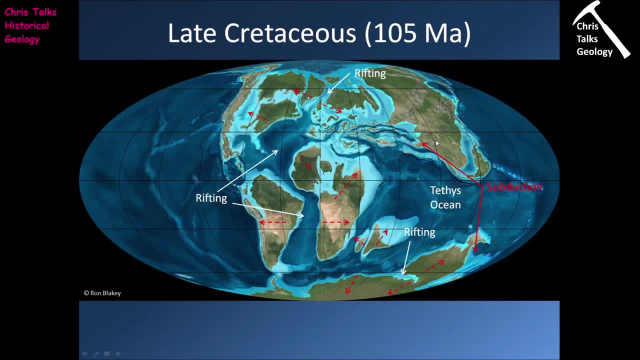 obviously helping to pull Africa northwards, helping to pull India northwards And, of course, this northward movement is achieved by subducting the Tethian Ocean seafloor underneath Asia And, of course, as I said, we're going to have a line of volcanic mountains. 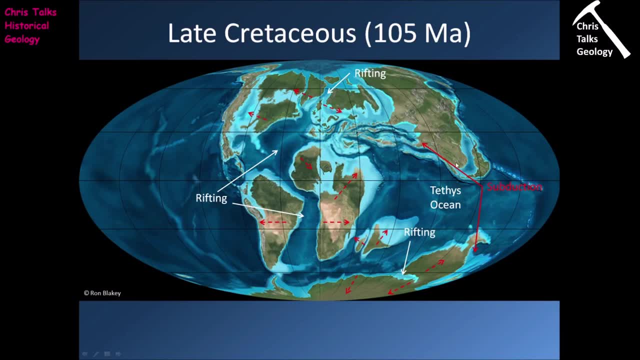 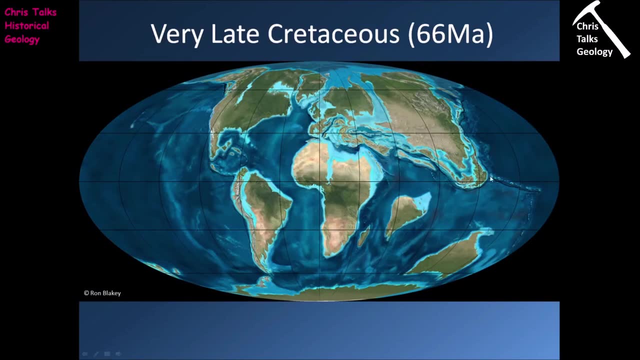 essentially here, along the southern margin of Asia, related to this ocean-continent subduction. Now what we're going to see is, as we move into the very late Cretaceous, India is making its way north. We still have the subduction zone operating here. 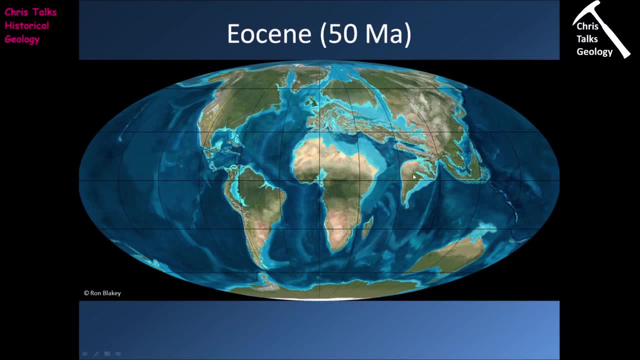 And then by the Eocene 50 million years ago. now, this is where India starts to decelerate. Here we go. This is India beginning to interact with Asia now, And this is helping to explain why India is now beginning to slow down. 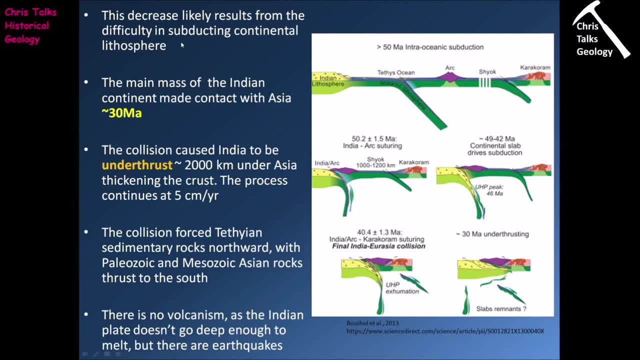 So, as I said, this decrease in velocity around 40 to 50 million years ago is going to be the result of the subducting, is going to be the result of the difficulty of subducting continental lithosphere, which essentially means you can't do it. 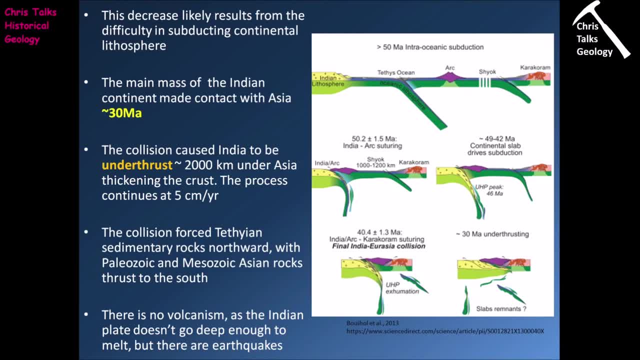 You can subduct oceanic crust, but subducting oceanic lithosphere is extremely difficult to impossible, And so this means that when you get two pieces of continental crust interacting with each other, all they can do is pretty much just plow headlong into each other. 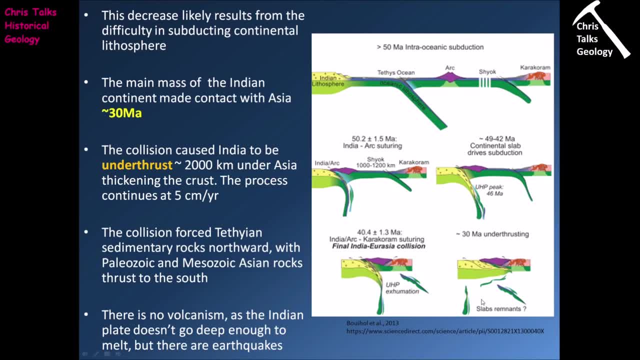 So if we look over here on this diagram we can see it kind of summarizes the processes that were taking place with regard to the Himalayan orogeny. So here's our situation. So we have India over here on the left, We have Asia over here on the right. 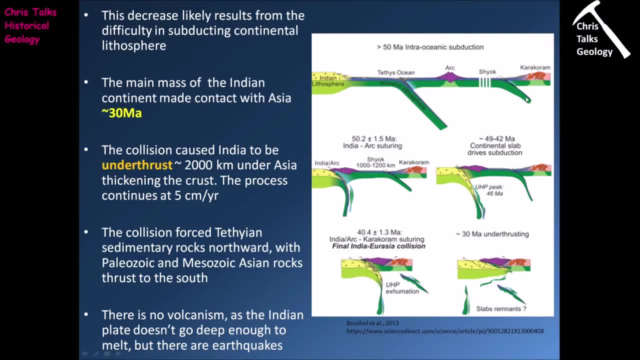 And you can see that we actually opened up two subduction zones. So the first subduction zone has the sea floor from the Tethian Ocean subducting underneath Asia And this leads to the formation of a volcanically active mountain chain along the southern margin of Asia. 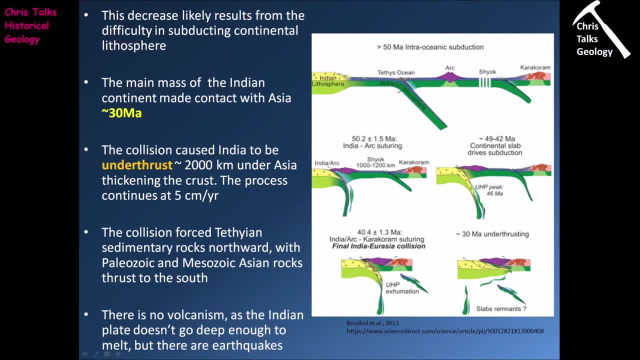 We also have another subduction zone opening up And this results in an ocean-ocean convergent plate boundary And it leads to the formation of a volcanic island arc system which sits in between Asia And India. So India is going to continue moving northwards as this bit of oceanic crust here gets subducted. 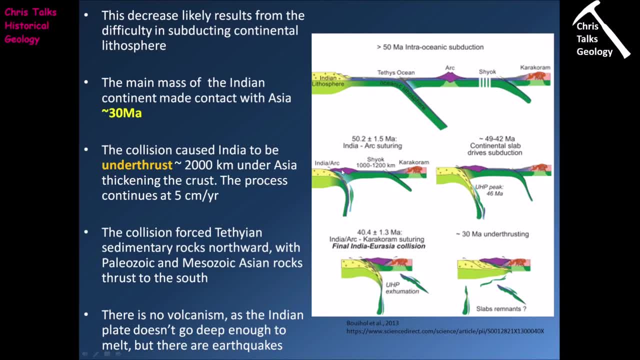 And that's eventually going to lead to the collision of India with this island arc about 50 million years ago, And this is the first indication of deformation that we see truly affecting the Indian continent Now, between 50 and 40 million years ago. we're really beginning to see India slow down. 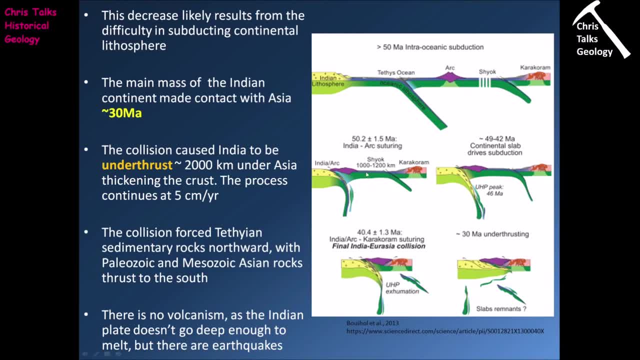 And you can see that's because this piece of oceanic crust here is being subducted. So we can see it's getting smaller and smaller And eventually about 40 million years ago. that's when we have India really beginning to interact now with Asia. 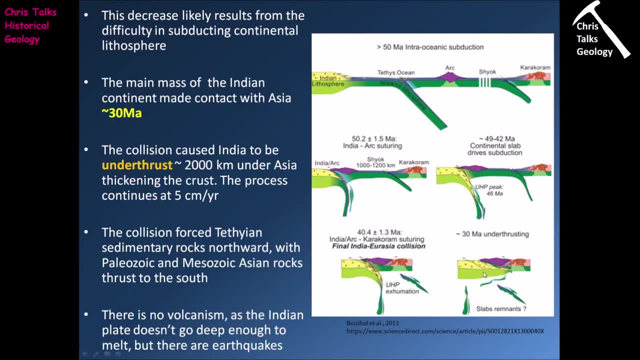 And then, about 30 million years ago, we have complete suturing of the two land masses together And the under-thrusting of the Indian continent underneath the Asian continent. Of course, this leads to a lot of crustal thickening and the formation of the Himalayan mountains. 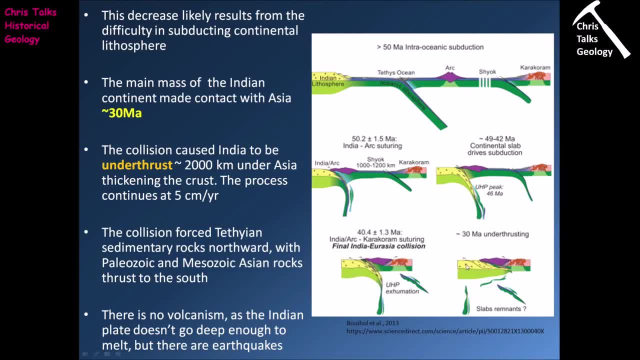 And the Tibetan plateau. So, in terms of this process of under-thrusting, well, this is simply the result of the fact that you can't subduct the continental lithosphere of the Indian continent. So when it hits the Asian continent, there's a few things that can happen. 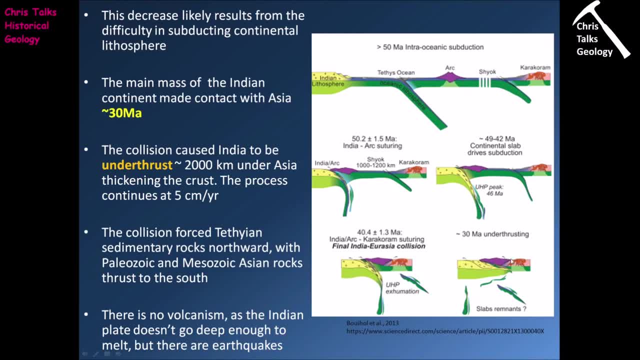 Even the Indian continent was going to go over the top of the Asian continent. It was going to go underneath the Asian continent, Or they were just going to crash head-on into each other And you know, neither of them was going to go over or under the top of the other. 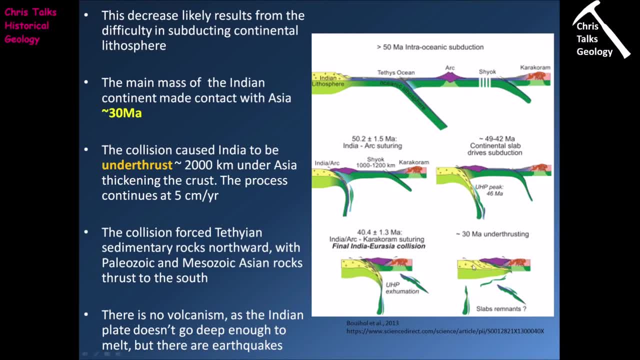 In this particular case, what we have is we have a situation where India got under-thrust underneath Asia And this essentially leads to approximately 2,000 kilometers of Indian continental crust being pushed along the bottom of the Asian continent, And this leads to obviously substantial thickening of the crust in this area. 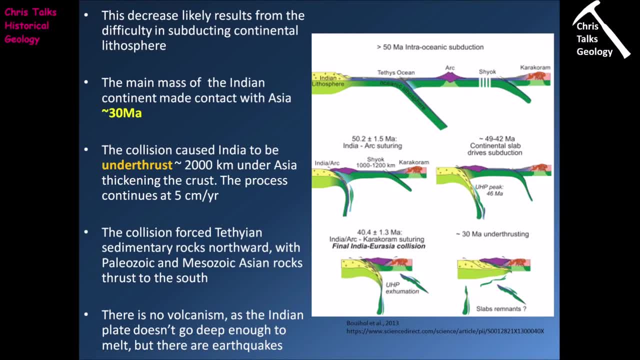 And of course that's expressed in the form of the Himalayan mountains. And this northward movement of India is still ongoing, And it's actually going on at 5 centimeters a year. It's still happening even now. So this orogeny isn't over yet. 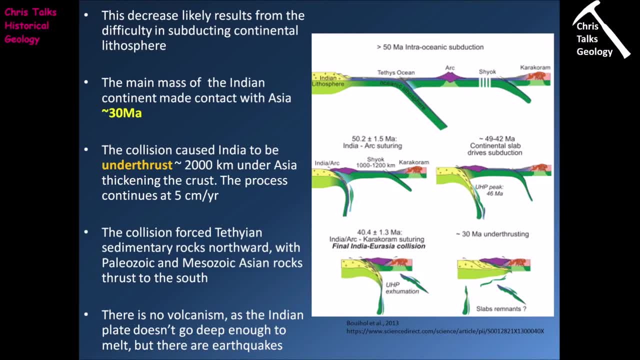 The Himalayan mountains are going to keep building and building until this northward movement stops. Now, as part of this collision, we have Tethian sedimentary rocks, Essentially so, that's rocks from the Tethian seafloor, And essentially these are all pushed northwards. 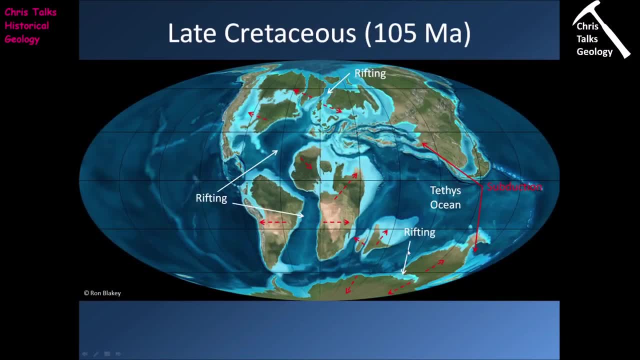 So, if you remember, if we just go back, we have all the rocks that were sitting here on the continental shelf of the northern continent And we have a large amount of sedimentary rocks here that will have been scraped off and will have formed an accretionary prism here. 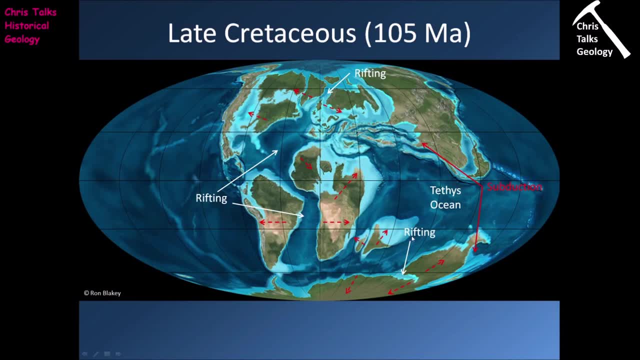 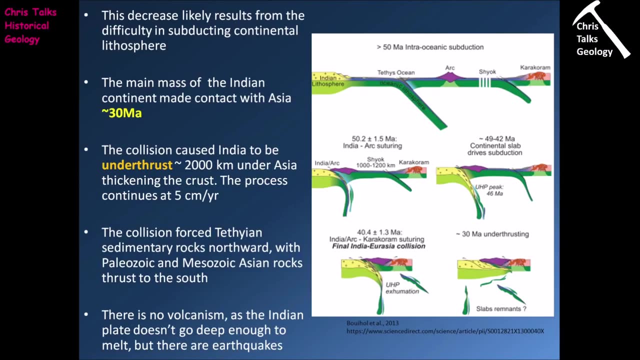 as part of this subduction zone. Well, all of those sedimentary rocks are going to essentially be mashed together by the collision And they're going to help to add mass to the formation of the Himalayan mountains In terms of Asian rocks. 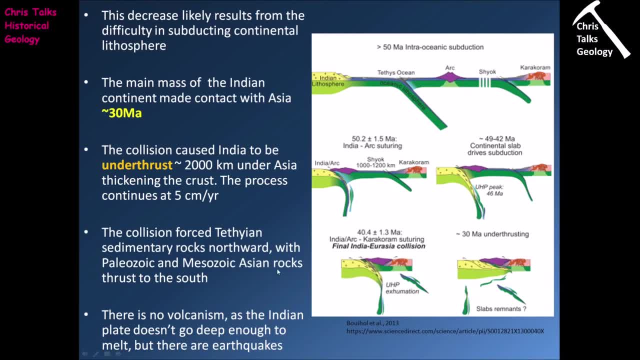 well, we have Paleozoic and Mesozoic Asian rocks which are being thrust south at the same time. So we have rocks related to the northward movement of India are pushed northward by the collision, And rocks related to the Asian continent. 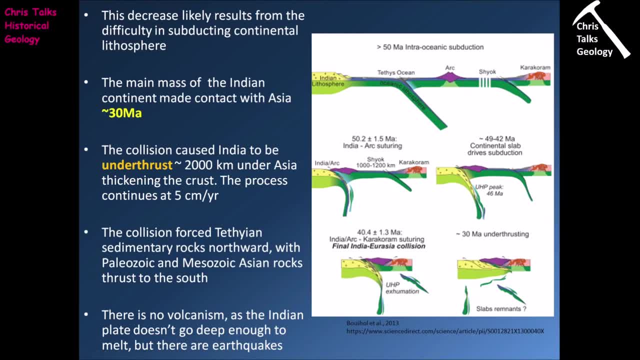 are at the same time being pushed south by the collision, So it's a bit of a messy situation In terms of the mountain range itself. the Himalayan mountains are, of course, not volcanically active, And this is because we don't have any subduction. 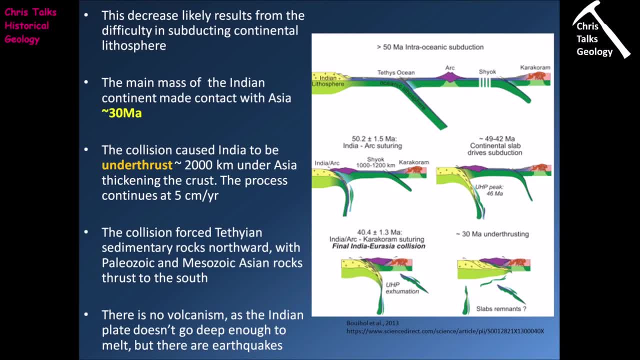 And if we don't have subduction, we don't have oceanic crust being pushed down into the mantle. Obviously, that oceanic crust therefore cannot dewater, So it can't cause mantle melting And of course, this will mean that we don't end up forming volcanoes. 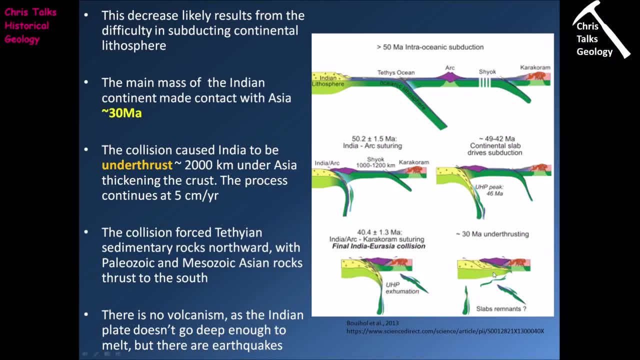 So the fact that we aren't pushing any kind of oceanic crust down into the mantle anymore means that volcanism in the area is going to stop. There is going to be some evening activity happening, And that's going to be right down at the base. 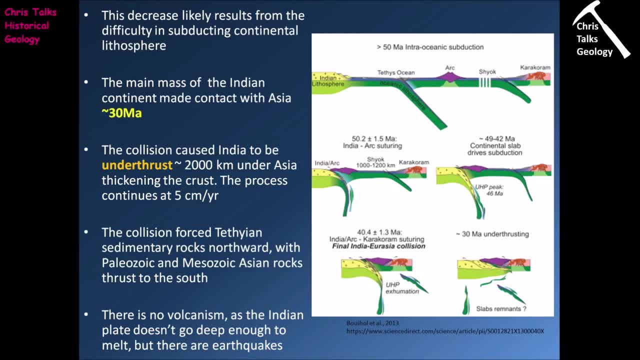 of the Himalayan mountain range, But this is not going to be related to any subduction process. This is related to the fact that we have all this crustal thickening taking place And this can lead to the melting of the continental crust at the base of the Himalayan mountains. 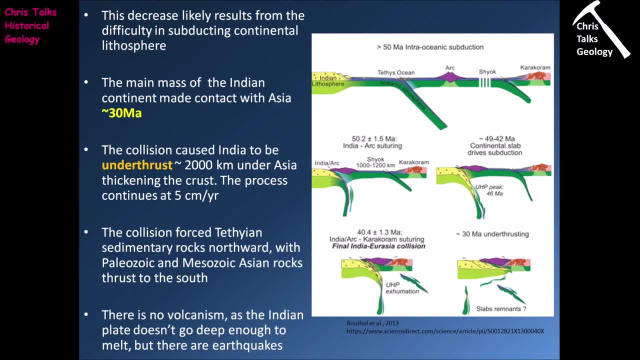 And so we can end up producing granites as part of this process. And so there are lots and lots of, you know, big granite intrusions forming as part of the Himalayan orogeny, But in terms of volcanoes it's very, very volcanically inactive. 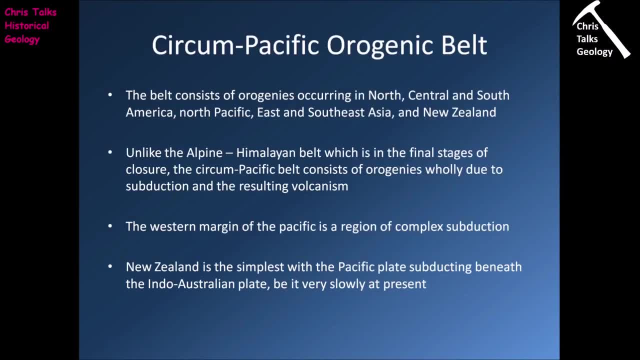 There's not much going on. Okay, so now let's think about the Circumpacific Orogenic Belt. So the belt consists of orogenies occurring along the North, Central and South Americas, North Pacific, East Pacific, Southeast Asia and New Zealand. 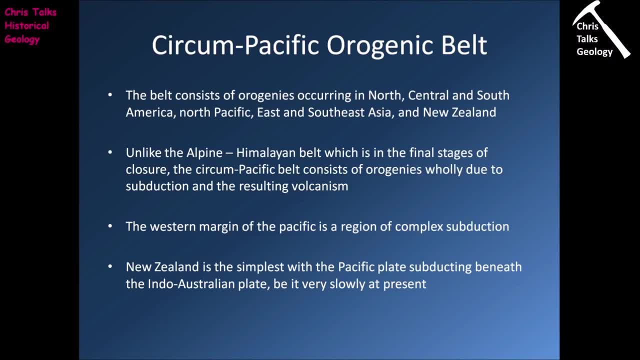 So it's a very extensive band of mountain building. Now, unlike the Alpine Himalayan Belt, which essentially is the final stages of a large-scale Wilson Cycle, the Circumpacific Belt consists of orogenies which are wholly due to subduction. 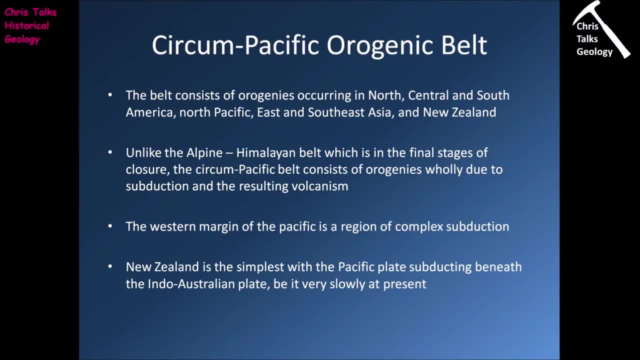 So ocean-ocean or ocean-continent subduction. So they're essentially part of the early stages of the closure of an ocean basin And, of course, as we've discussed, the fact we have oceanic crusts subducting down into the mantle. 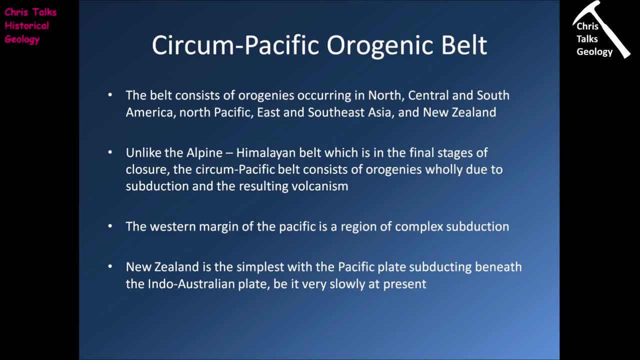 means we have the capacity to form quite a lot of magma. So obviously that means these mountain ranges associated with the Circumpacific Orogenic Belt are going to be very volcanically active, And so this is why the Circumpacific Orogenic Belt 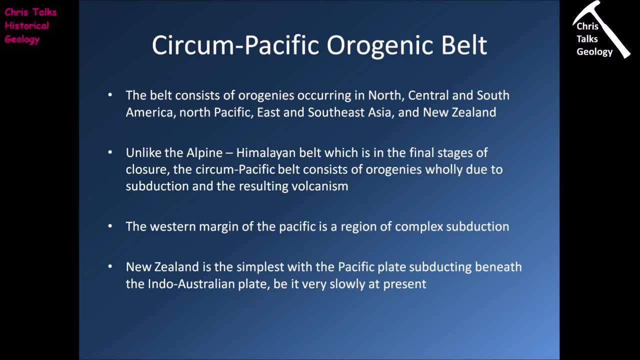 is sometimes referred to as the Ring of Fire, because there are so many volcanoes. Now the western margin of the Pacific is a region of rather complex subduction And we're going to run through that. There's a lot of stuff going on. 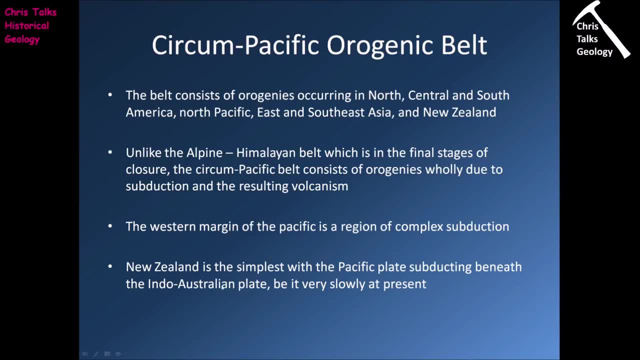 In terms of the simplest portions of the Circumpacific Belt. the simplest portion is around New Zealand And in this area we have the Pacific Plate subducting beneath the Indo-Australian Plate, be it very, very slowly. So in that area we can see what's going on quite easily. 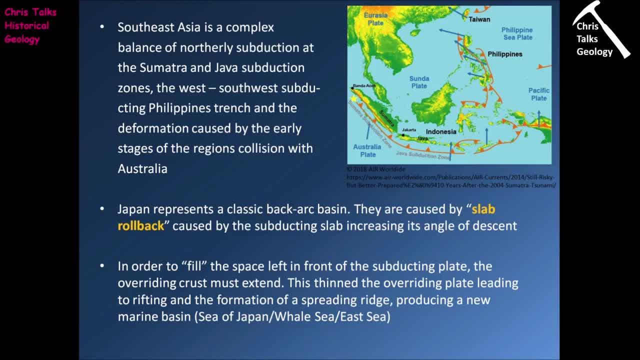 Now, in terms of Southeast Asia, the subduction process is extremely complicated. Now this is because we actually have two major orogenic events operating in the same area. So if we look here we can see we have the Sumatran and Javan Trenches. 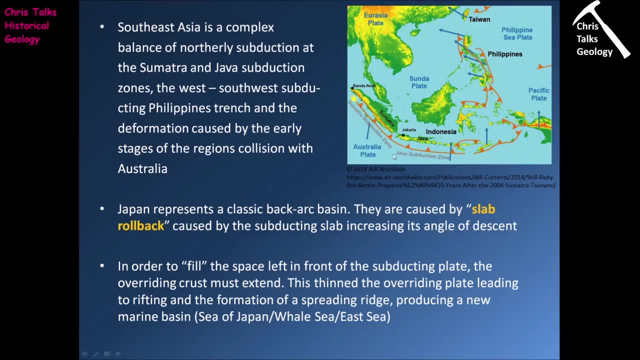 running along the southern edge of Indonesia. Of course, these are related to the Northward Movement of Australia And so these are, you know, to want of a better way of describing it, considered to be part of the Alpine Himalayan Orogeny. 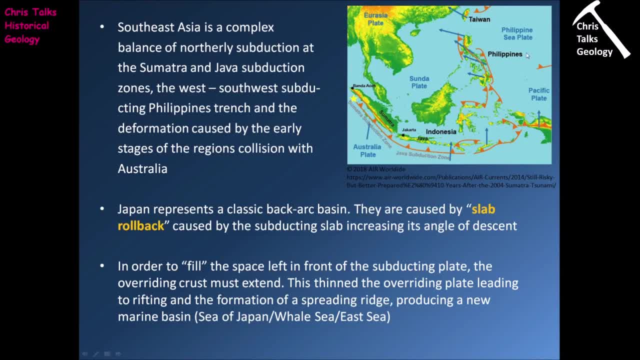 Over here in the northeast of the image we can see, we have a number of trenches related to the subduction of the Philippines Plate underneath the Eurasian Plate, And so we have two major orogenies: one essentially moving across northwards from the south. 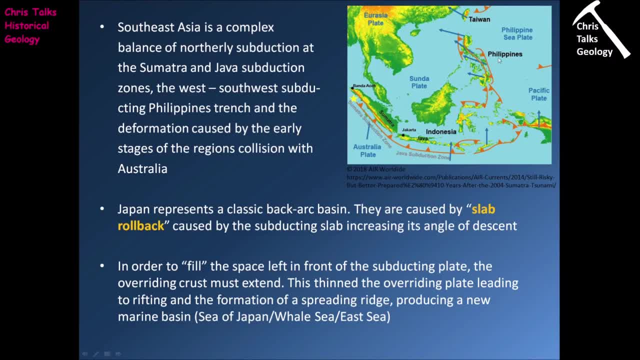 and one moving across westwards from the east. So Southeast Asia is a complex balance of northerly subduction and westerly subduction And this means essentially you have a very, very complex situation And you can see that by the you know. 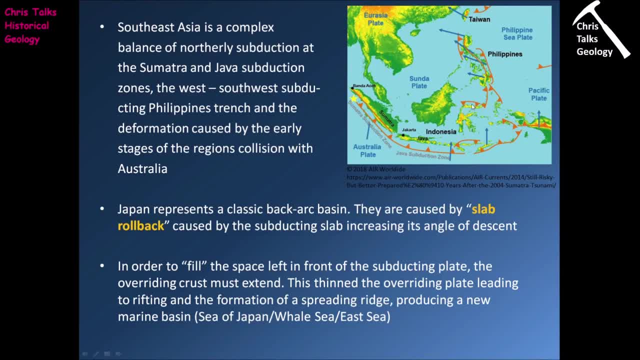 the amount of small subduction zones operating in this area. So you know this explains why this situation is so complex. This explains why this area, Indonesia, the Philippines especially, are so tectonically and volcanically active, because there's a lot going on there. 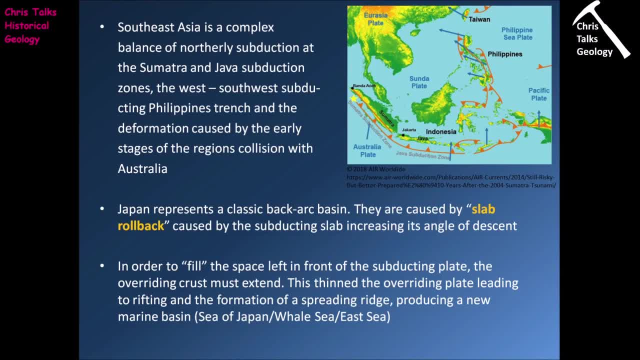 There's lots of subduction processes. That means lots of magma being produced. obviously, All the pressure being put into this area by these two convergent events are also going to mean the rocks are, you know, going to be under a lot of stress. 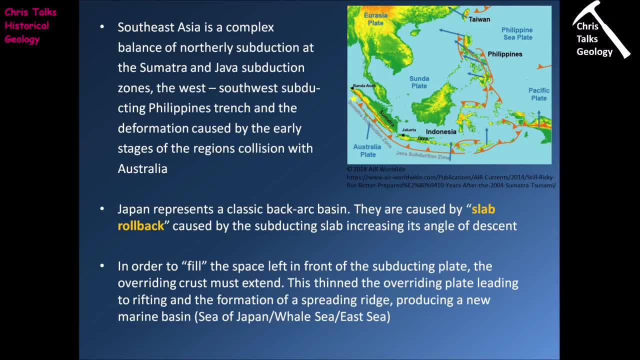 They're going to be very, very heavily deformed, And so this means in this area, earthquakes and volcanic activity are going to be very, very likely. Now, in terms of Japan, if we were to go further up the coast, 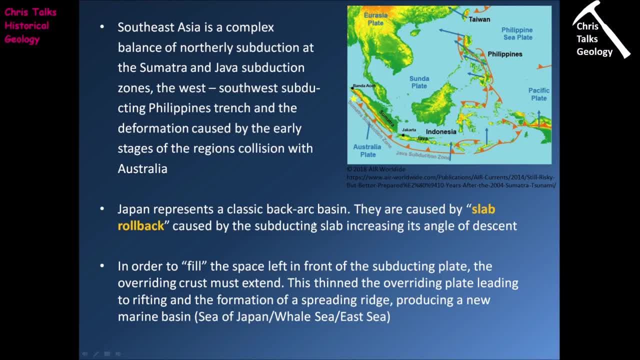 Japan represents a classic back-arc basin situation, And so the formation of this back-arc basin is probably the result of what's referred to as slab rollback, And you might remember this term from earlier presentations. So all slab rollback is is we have a piece of subducting oceanic crust. 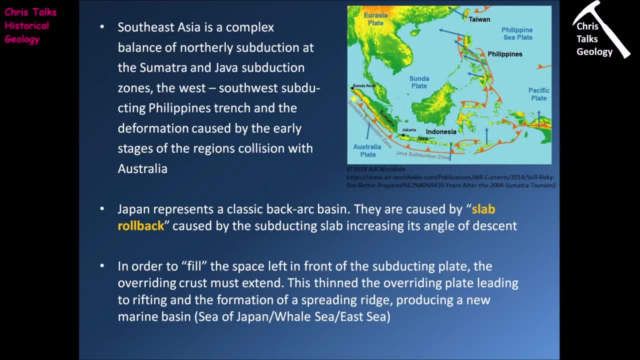 And let's say, for instance, it's subducting down into the mantle at 45 degrees. Well, let's say, over time, the angle of subduction steepens up. It goes from 45 to, let's say, 75 degrees. 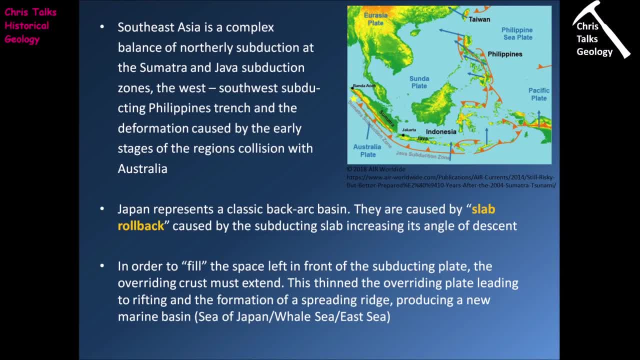 So now the oceanic crust is diving down into the mantle at a much higher angle. Well, what this means is, as the oceanic crust rolls backwards and, you know, begins to take up this higher angle of subduction, it means a small gap begins to open up. essentially, 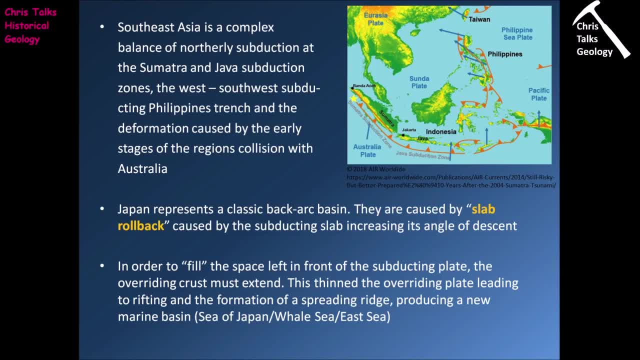 between the subducting oceanic crust and the continental crust, that's going over the top of it. And so what happens is, is the continental crust or oceanic crust overriding over the top, has to extend to fill the space, So it begins to stretch. 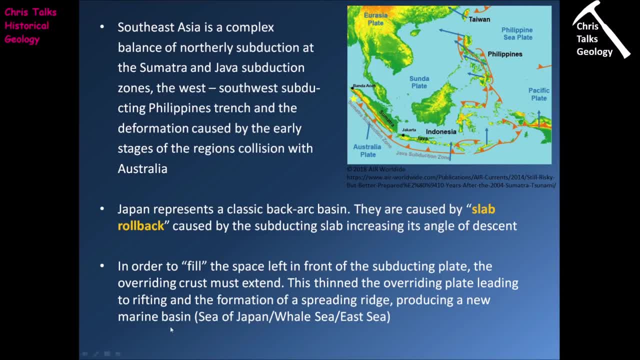 And so this can result in the crust becoming thinner, And then that means the overriding plate, so the crust of the overriding plate becomes thinner, This can eventually obviously form a rift valley, And if the rift valley continues and becomes, you know well enough, developed, 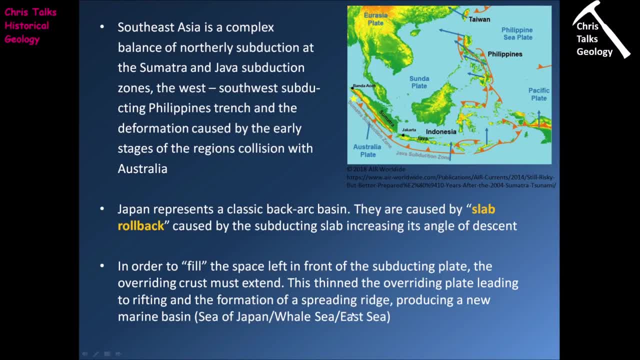 it can lead to the formation of a spreading ridge due to decompressional melting of the mantle- And this is exactly the process we see with Japan- And this back arc basin goes to form the well, depending on how you want to name it. 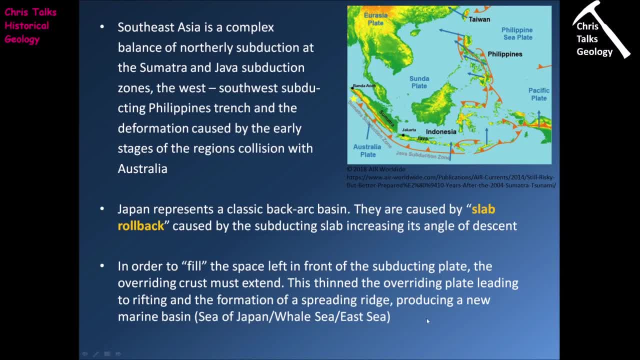 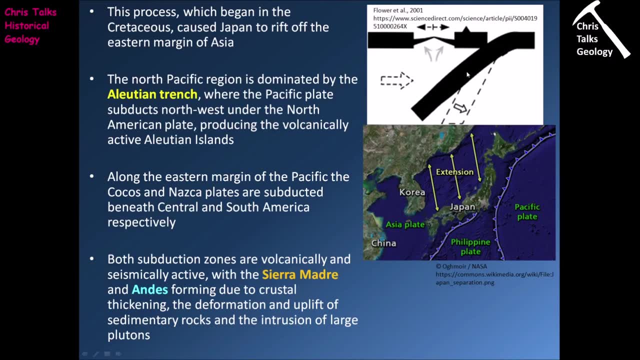 you can even call it the Sea of Japan, the Whale Sea or the East Sea. So here's our situation for Japan. So here's our subduction zone. We have our oceanic crust subducting down here and we have our continental crust here. 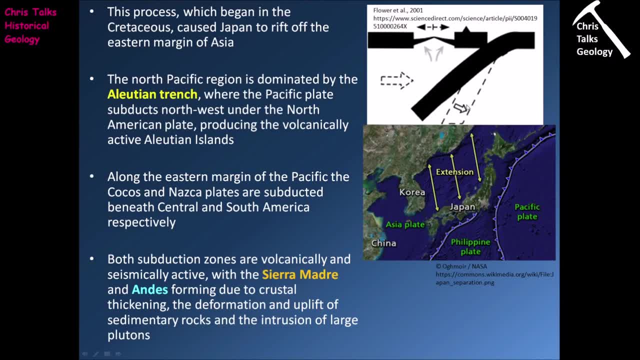 In the case of slab rollback, the angle of subduction increases And this means we end up, you know, opening up a gap at the front. In order to fill that gap at the front, the continental crust has to extend And this leads to an area of the continental crust. 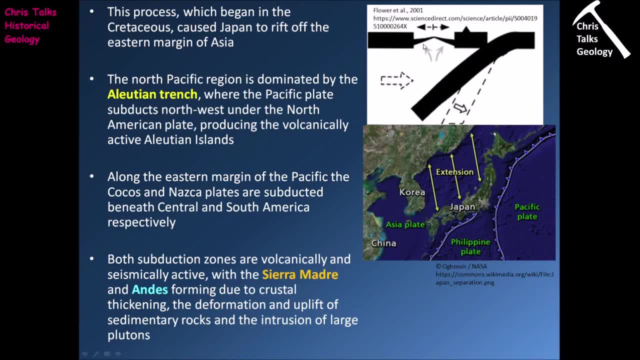 which will begin to rift. It will become thinner And eventually, if it becomes thin enough, it can lead to decompressional melting of the mantle underneath And of course, at that point we start producing large quantities of mafic magma. 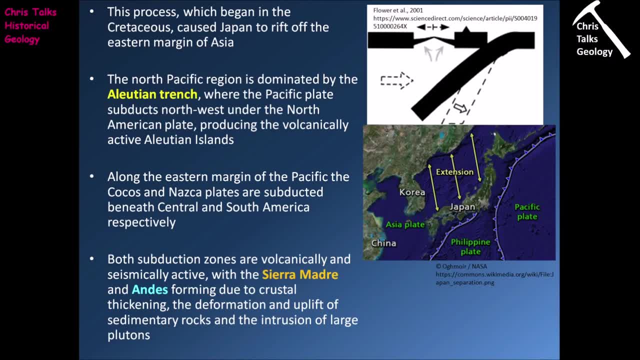 That's going to make its way to the surface and it's going to form oceanic crust, And so we're going to end up forming an ocean basin, And that's exactly what we can see here. So here's the basin itself, And we can see if you actually look at Japan. 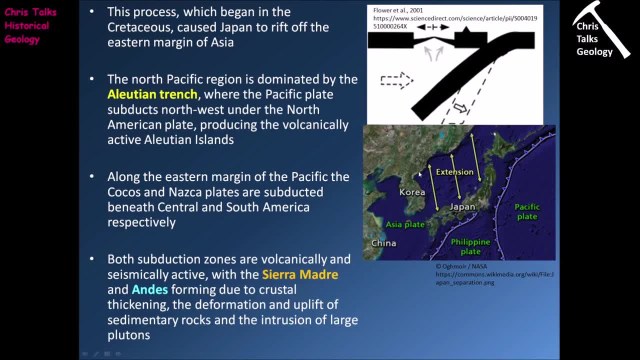 and you were to move it northwards, you would actually see that Japan would link quite comfortably onto the edge of Asia here, And so what's happening is here, our subduction zones. we've had slab rollback that's led to extension in this area. 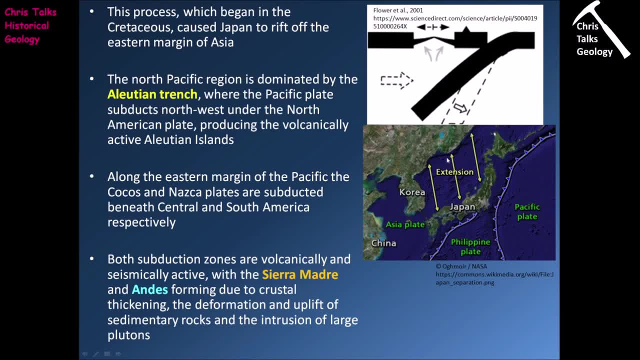 And essentially it's led to Japan being pulled off the side of Asia in a southerly direction, And the space in between has been filled up through the production of new oceanic crust In terms of the northern margin of the circum-pacific belt. 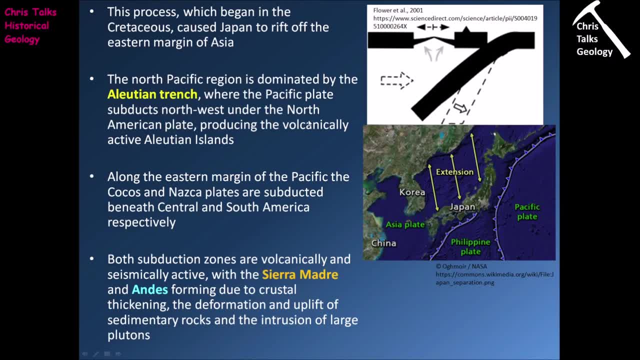 well, that's dominated by the Aleutian Trench. So that's where the Pacific Plate is subducting in an approximately northwesterly direction under the North American Plate, And it's produced the very volcanically active Aleutian Islands. 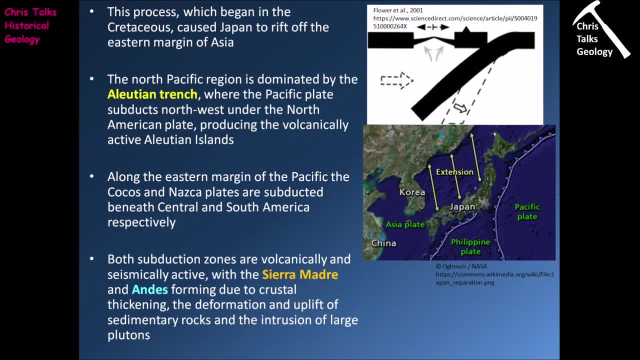 It's kind of the classic example of an ocean-ocean convergent plate boundary. Now, along the eastern margin of the circum-pacific belt, we have the Cocos Plate and the Nazca Plate subducting beneath Central and South America respectively. 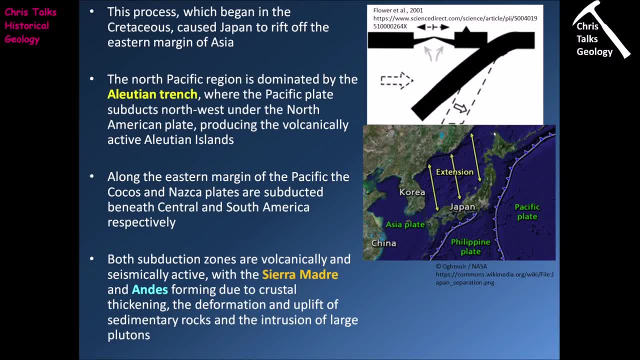 Both of these are classic examples of ocean-continent subduction. So we end up forming large, volcanically active mountain ranges which are also very, very prone to earthquakes, as you would expect. Both subduction zones, both the subduction zones related to the Cocos.